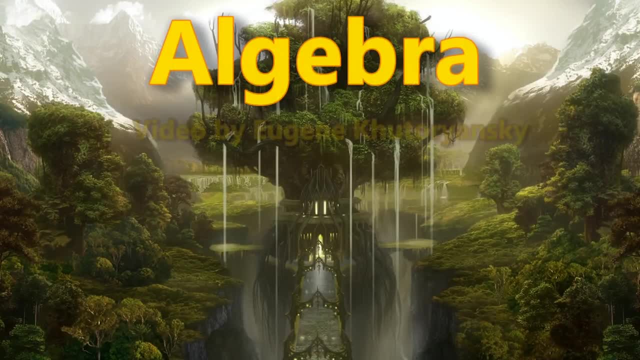 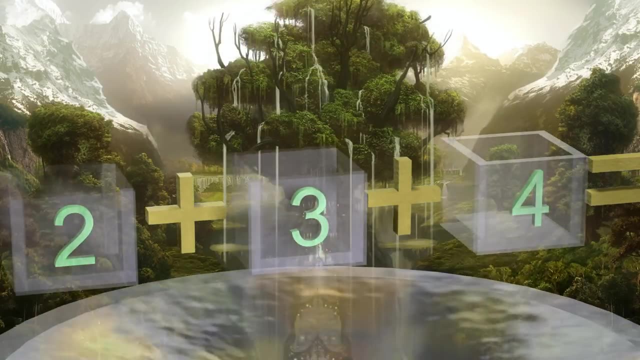 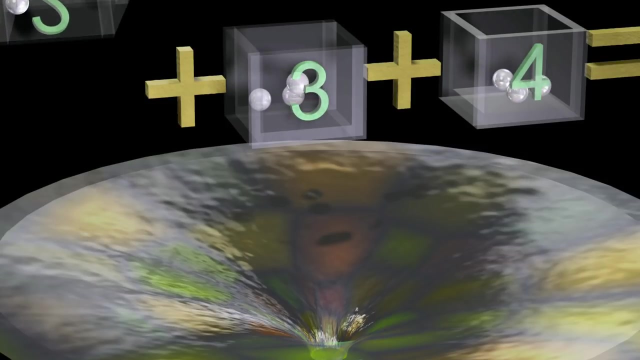 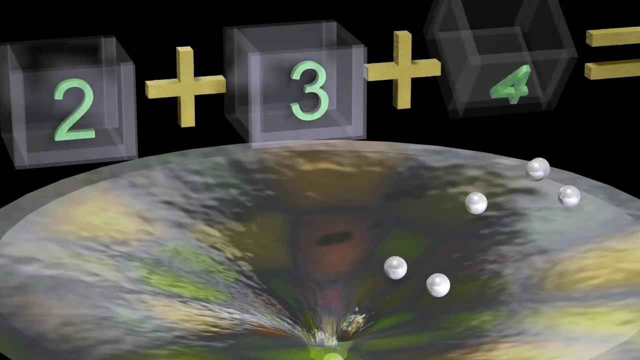 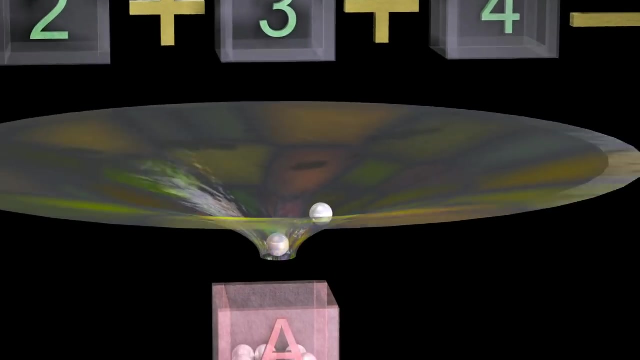 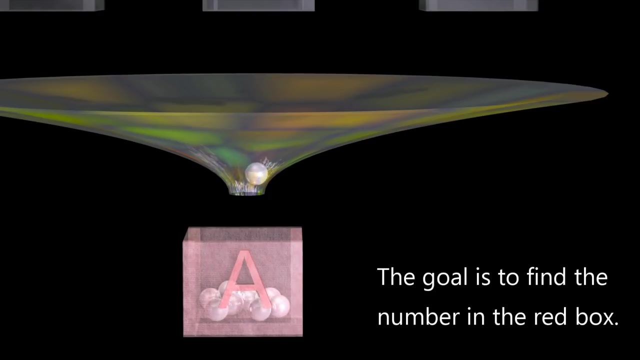 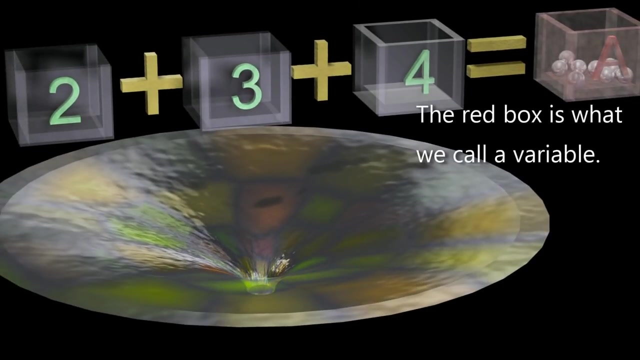 Algebra is the foundation of all science and technology. Algebra is the foundation of economics and engineering. Algebra is a key to understanding logic and everything in the world around us. The goal is to find the number in the red box. The red box is what we call a variable. 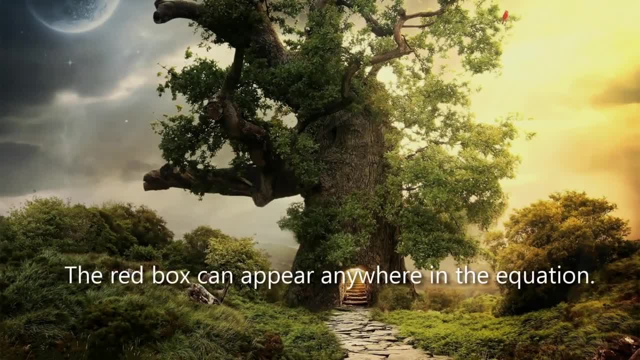 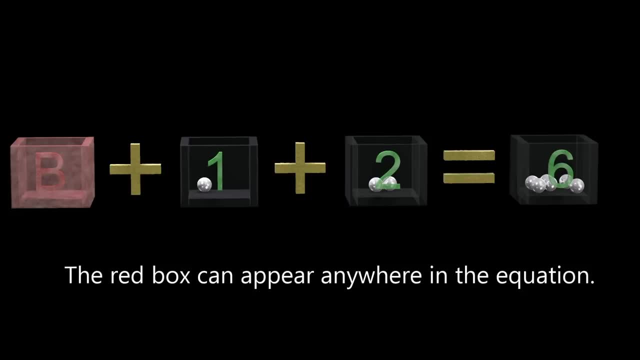 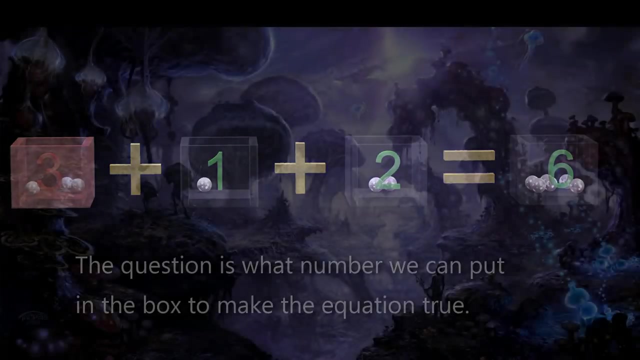 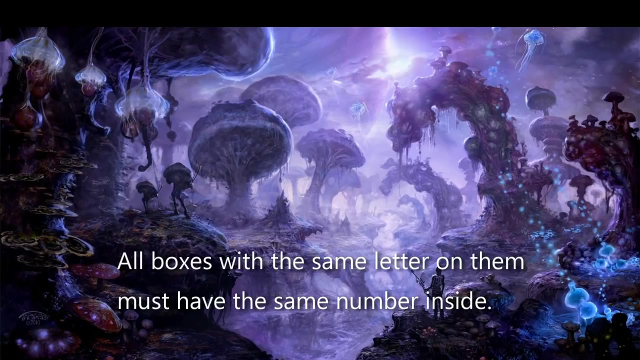 The red box can appear anywhere in the equation. The question is: what number can we put in the box to make the equation true? All boxes with the same letter on them must have the same number. All boxes with the same letter on them must have the same number inside. 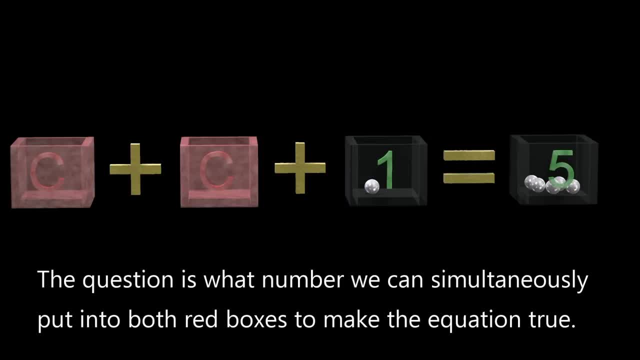 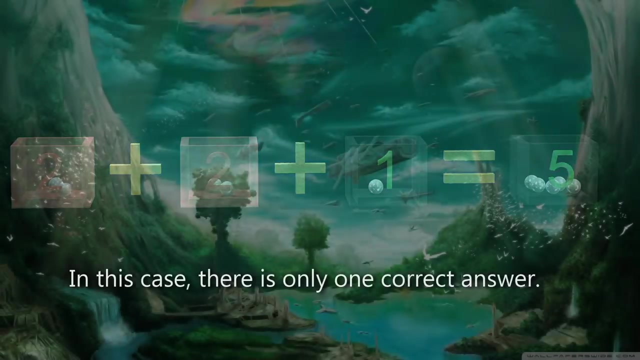 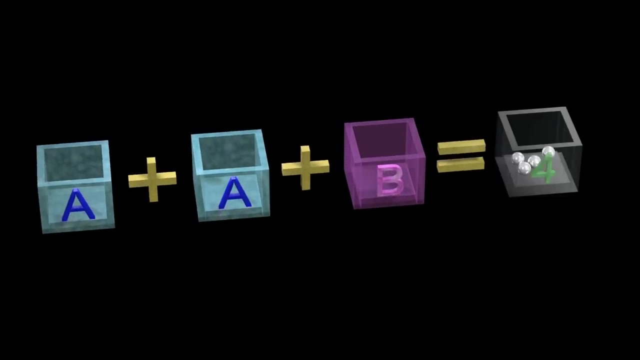 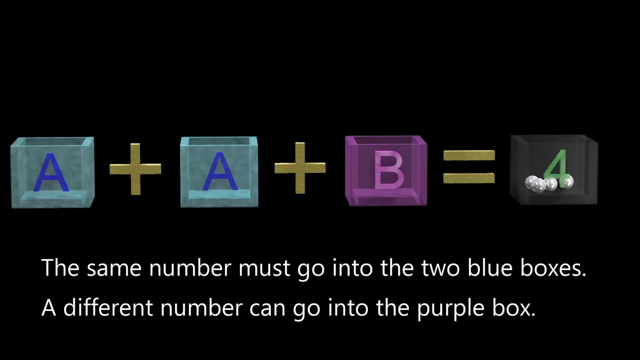 The question is: what number can we simultaneously put into both red boxes to make the equation true In this case? In this case, one correct answer: The same number must go into the two blue boxes. A different number can go into the purple box. 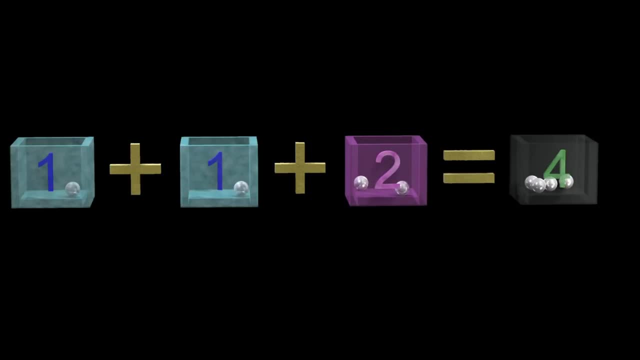 In this case. In this case there are many correct answers. Life rarely has only one variable. Life rarely has only one variable Here. Here, the two blue boxes are one variable. Here, the two blue boxes are one variable. The purple box is a second variable. 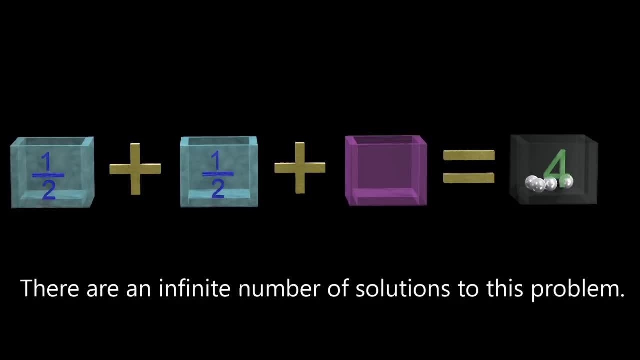 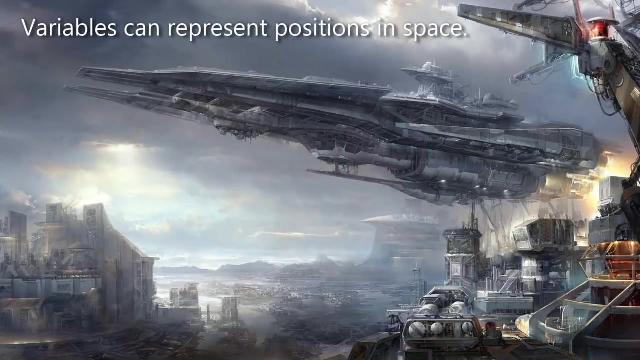 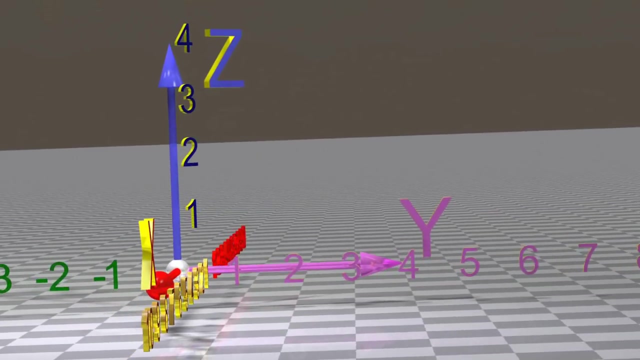 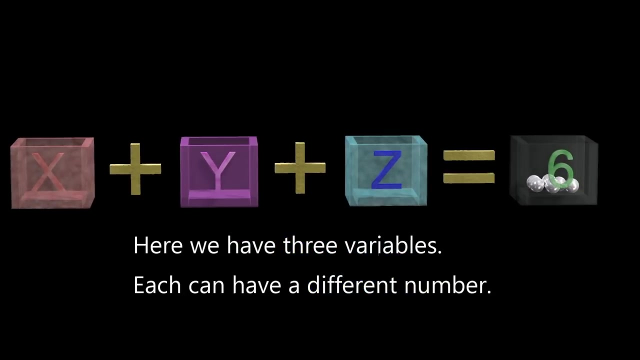 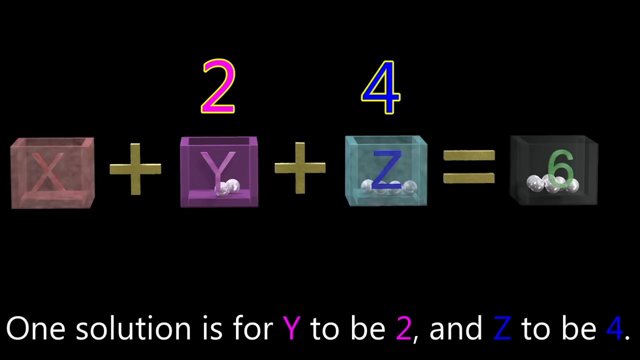 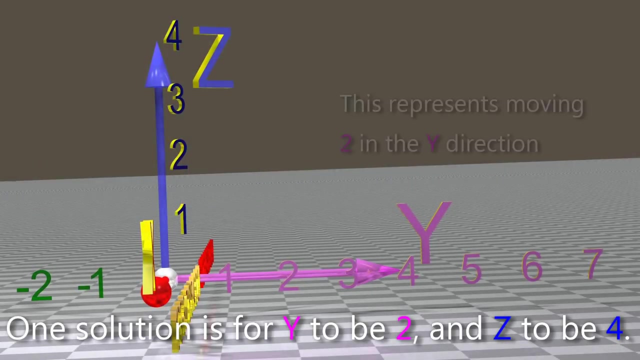 There are an infinite number of solutions to this problem. Variables can represent positions in space. Here we have three variables. Each can have a different number. One solution is for y to be 2. And for z to be 4.. This represents moving 2 in the y direction. 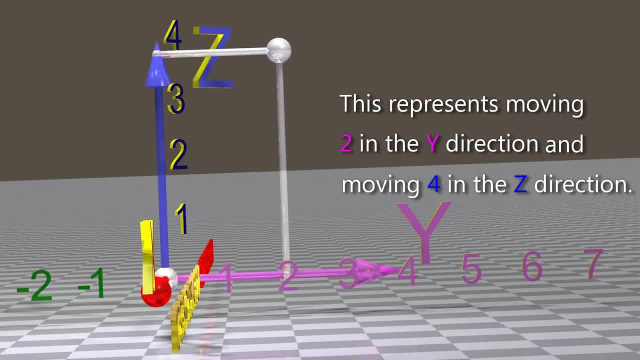 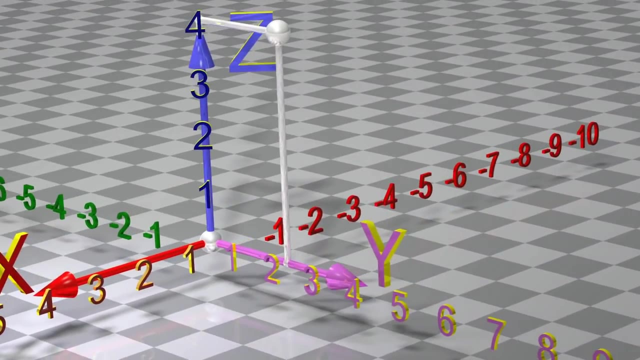 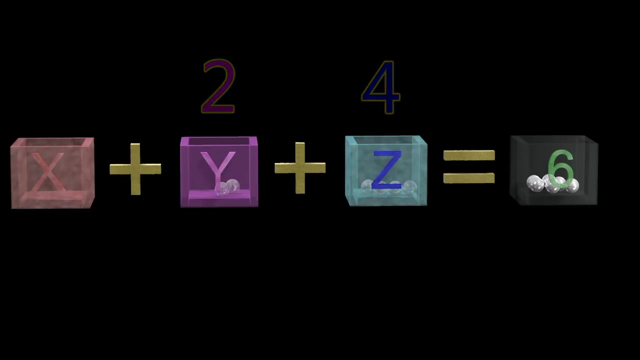 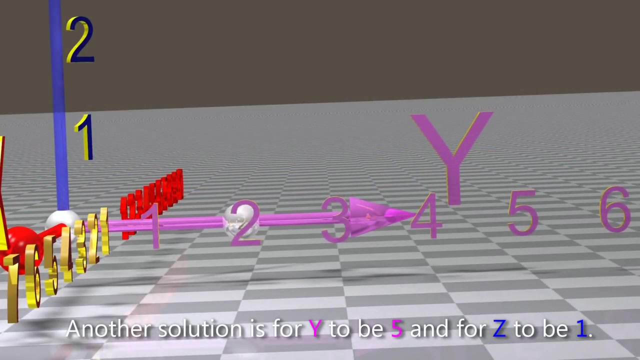 And moving 4 in the z direction. Another solution is for y to be 5. And for z to be 1.. This represents moving 2 in the y direction And moving 4 in the z direction. This represents moving 4 in the y direction. 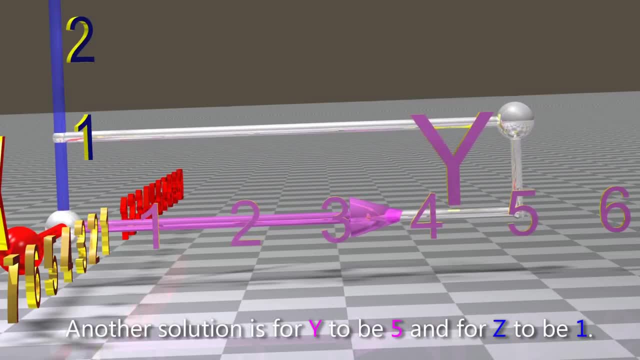 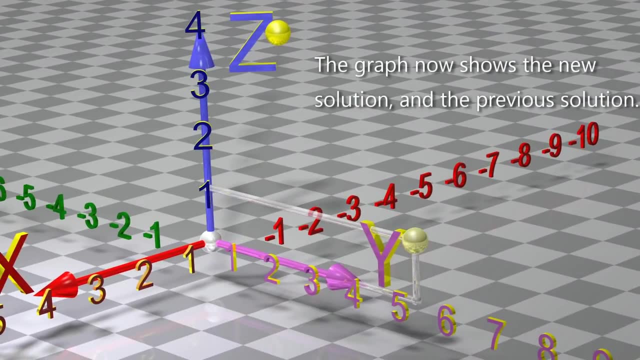 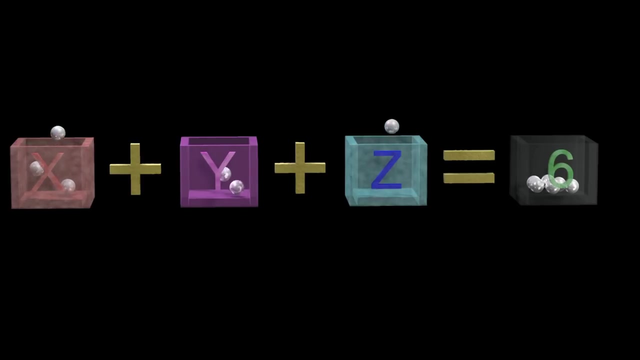 And moving 4 in the z direction. The graph now shows the new solution and the previous solution. The graph now shows the new solution and the previous solution. Another solution is for x to be 3.. For y to be 2. And for z to be 1.. 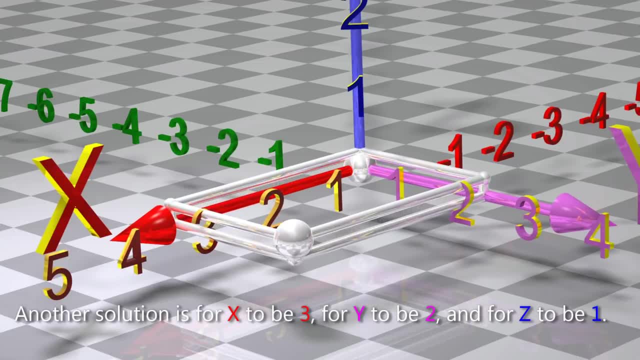 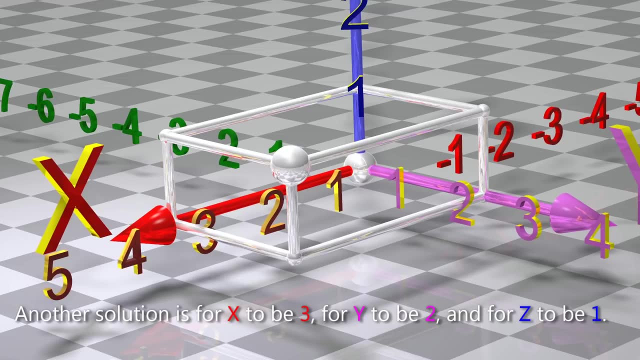 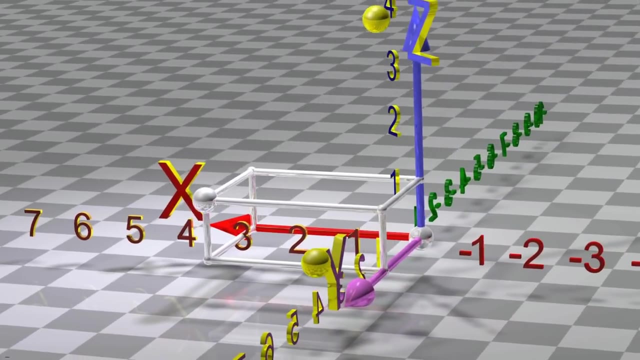 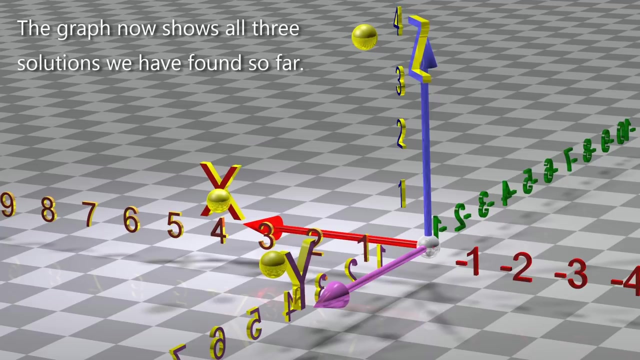 The graph now shows the new solution and the previous solution For z to be 2.. For y to be 2: The graph now shows all three solutions we have found so far. The graph now shows all three solutions we have found so far. 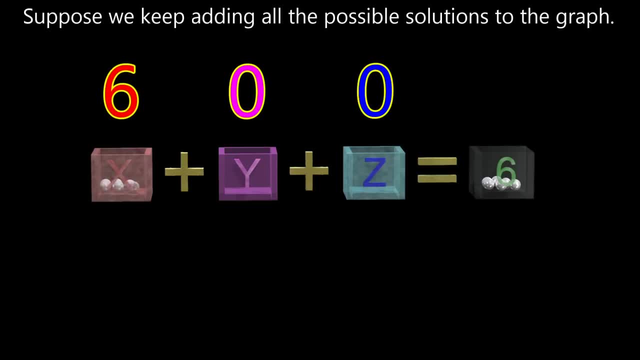 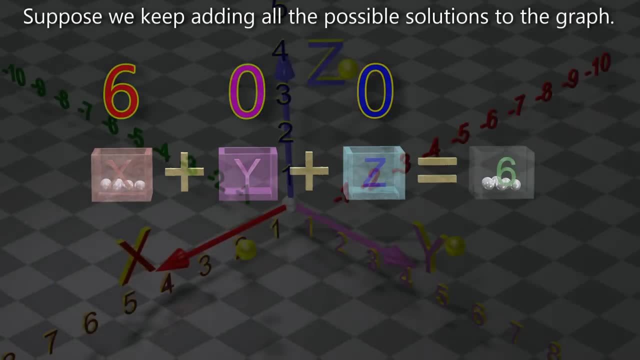 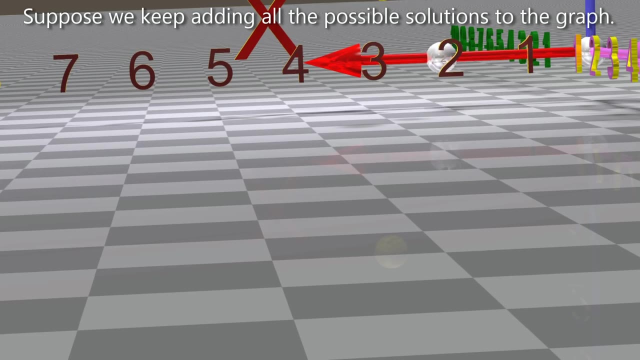 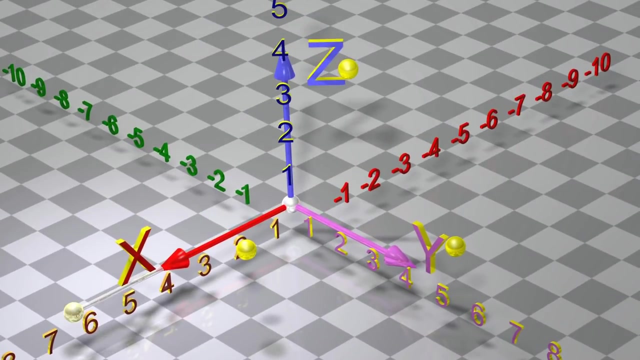 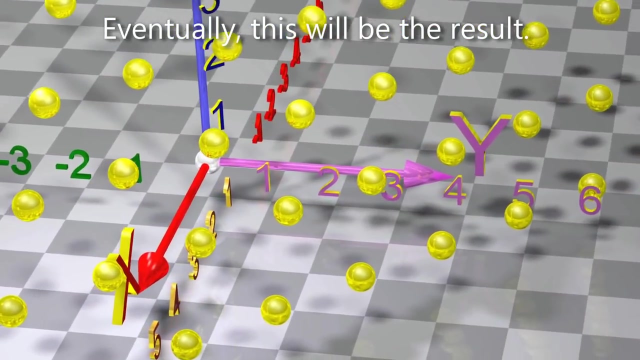 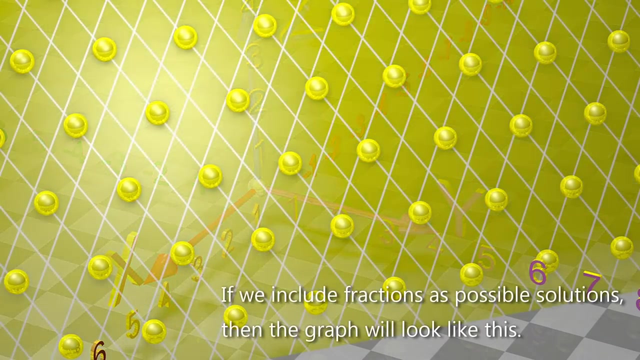 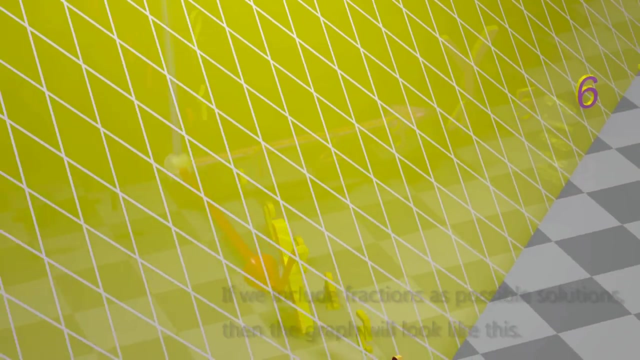 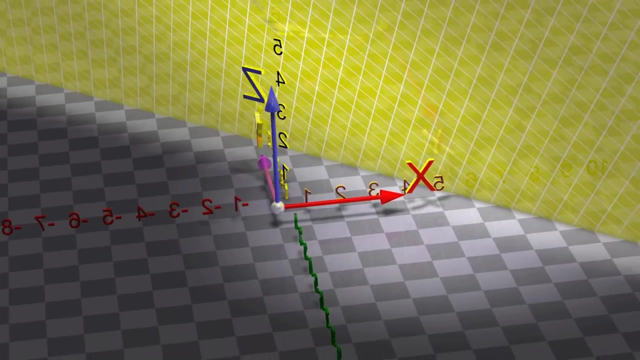 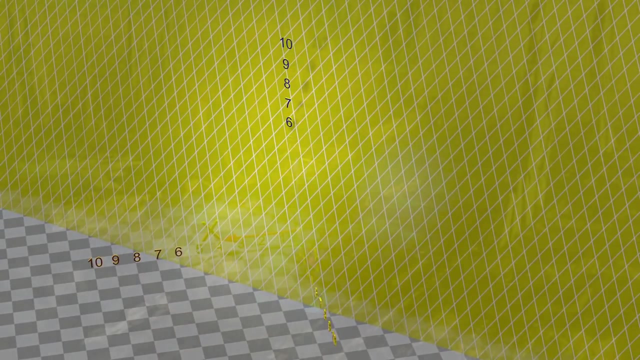 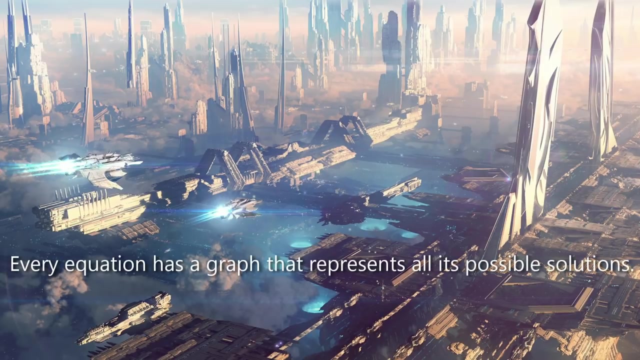 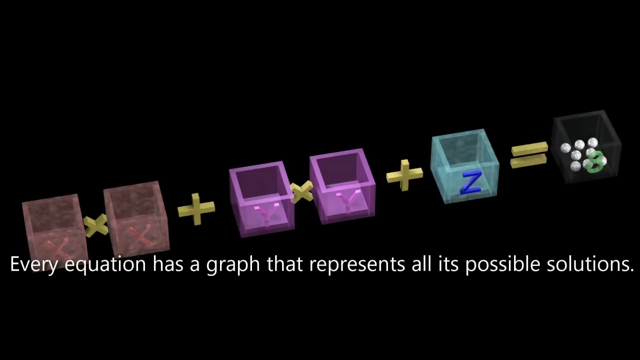 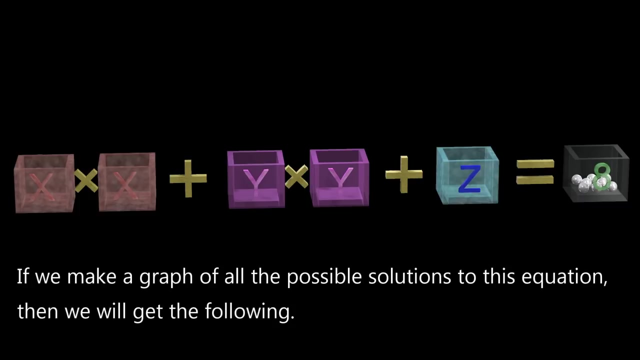 Suppose we keep adding all the possible solutions to the graph. Eventually, this will be the result. If we include fractions as possible solutions, then the graph will look like this: Every equation has a graph that represents all its possible solutions. If we make a graph of all the possible solutions to this equation, 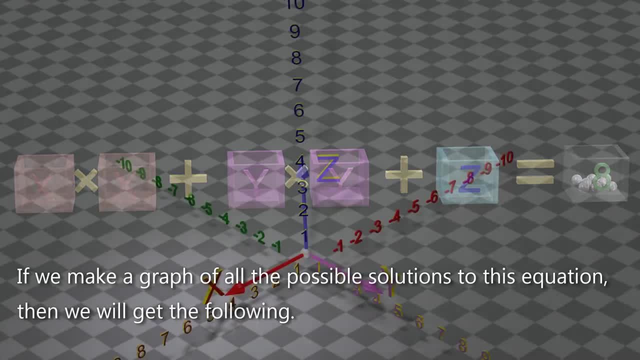 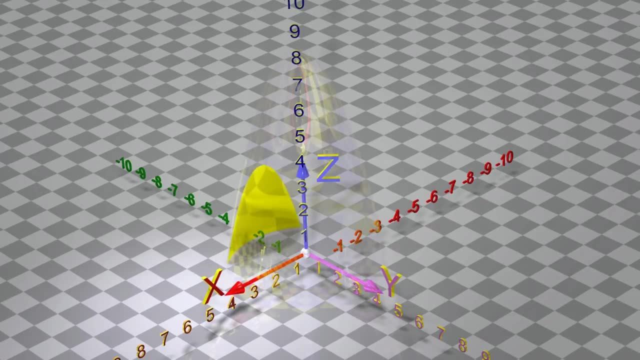 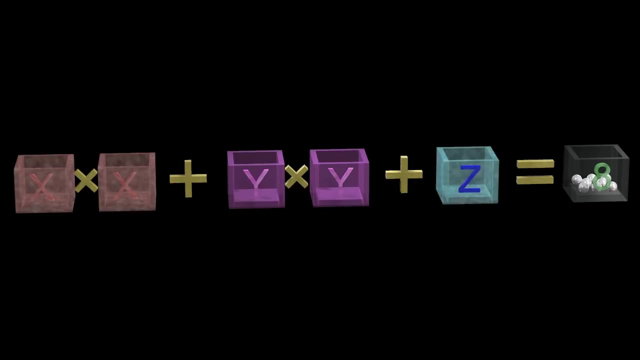 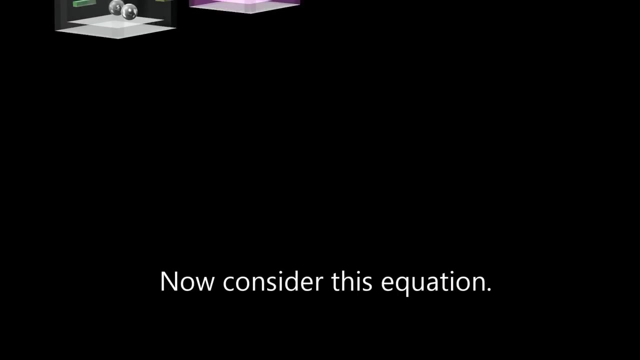 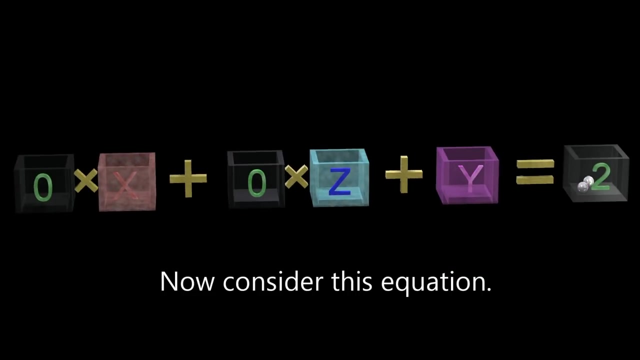 If we make a graph of all the possible solutions to this equation, then we'll get the following. Now consider this equation. This is one possible solution, And so is this, And so is this, Since zero multiplied by any number is zero. 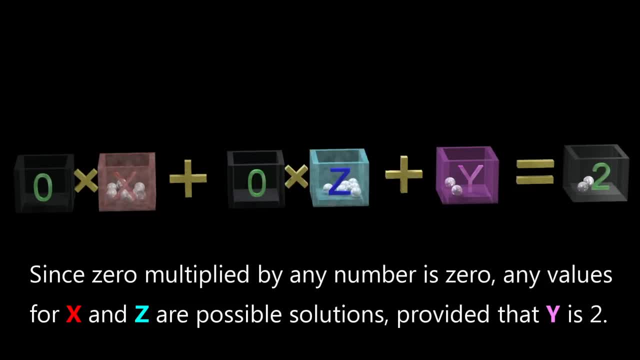 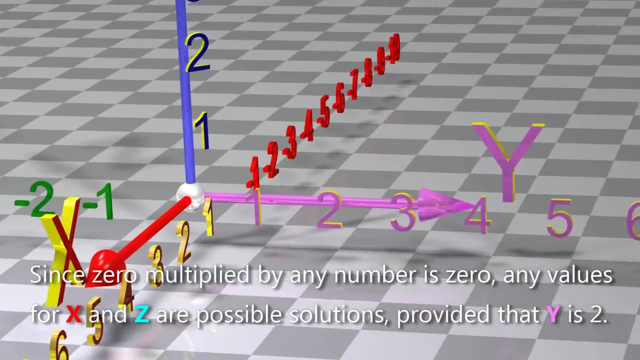 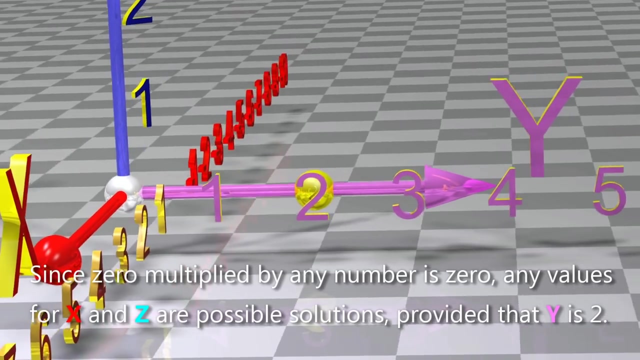 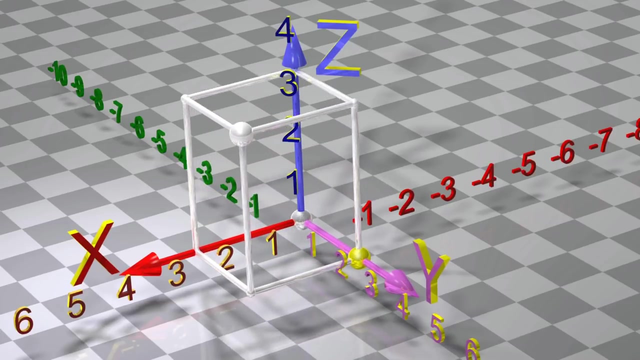 Any values for x and z are possible solutions, provided that y is two. Any values for x and z are possible solutions provided that y is two. Any values for y and z are possible solutions provided that y is two And these numbers arefish Incredibles. 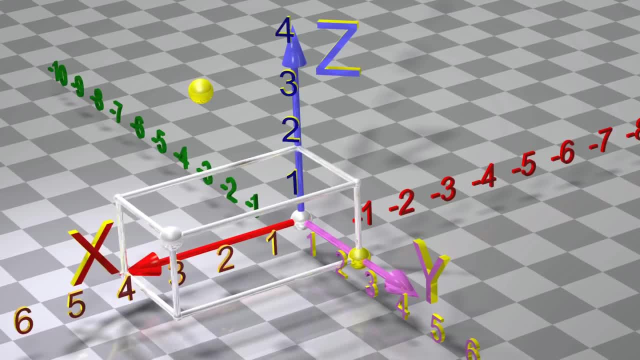 and h. we make zero shrimp grandchildren: 0, 1,2,, 0,, 3, 4.. 0, 1,2,, 2,, 3, 4.. To make a zero mean zero: 0,, 1,2,, 0, 3.. 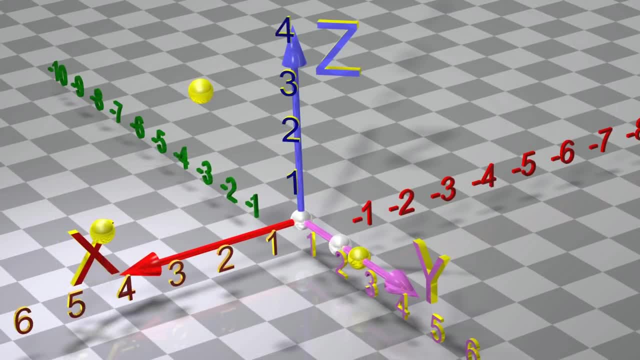 0,, 1,2,, 2,, 3,, 4.. Now, what we'll do? Now, what we've just done is we're working with numbers. What are the initial�를? maturity rate revenue. 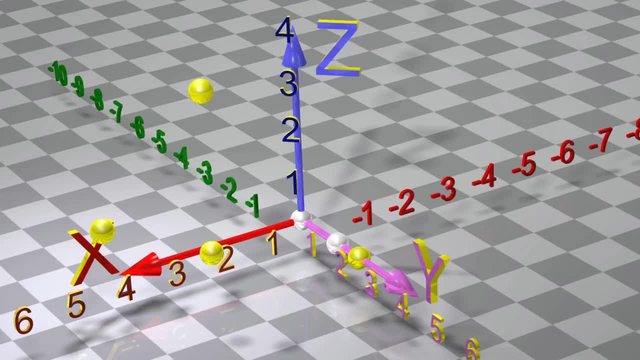 150,000, Dan. Welcome everyone to Hana World. You've been listening to Mana Research. I'm Sandy Lubous. This video was made possible by the information on this programme. Then there's going to be more information about companies that weilff time and in thece. 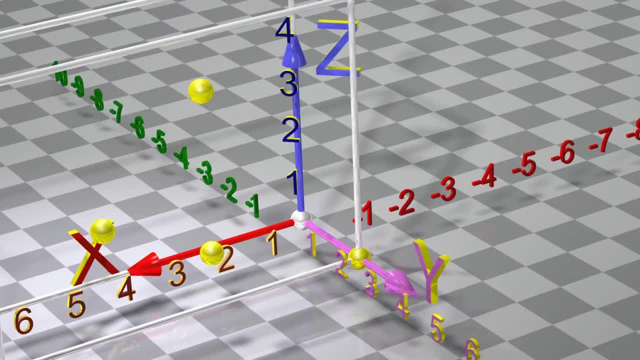 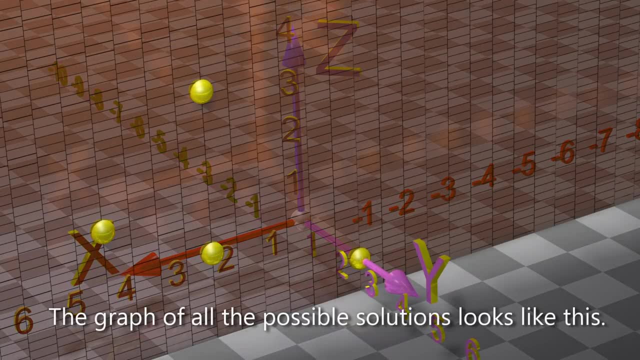 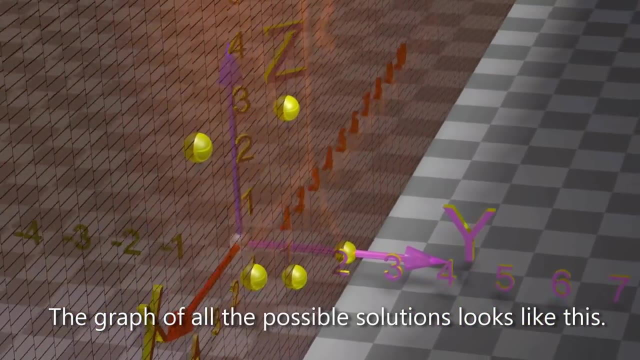 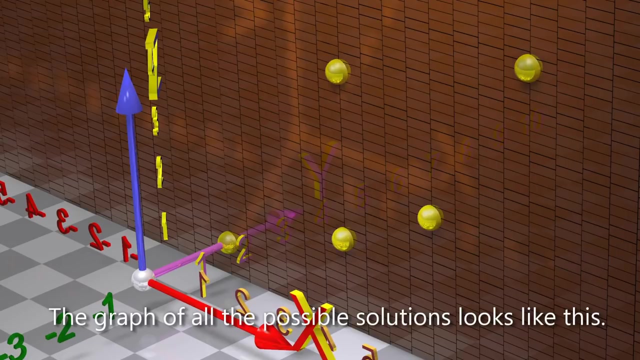 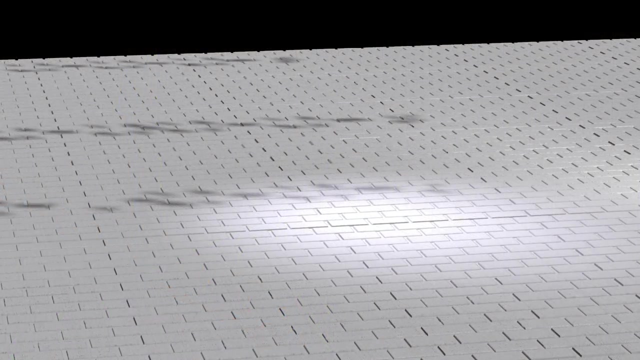 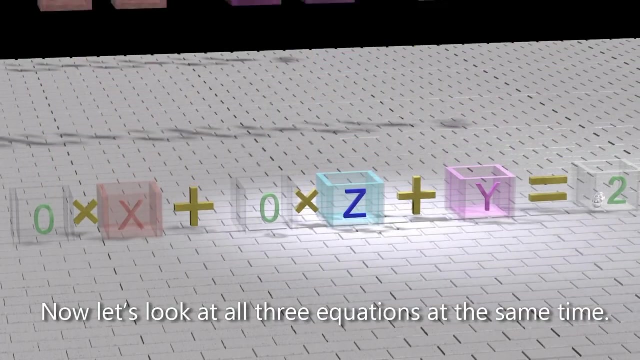 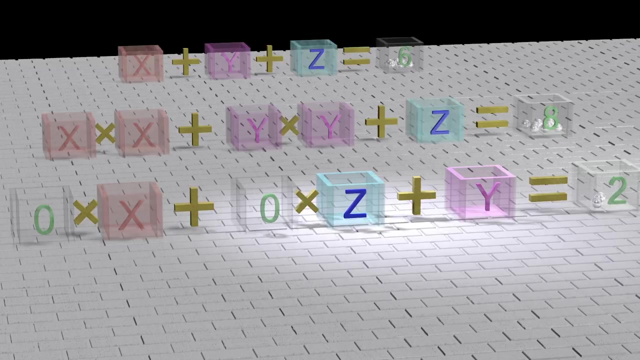 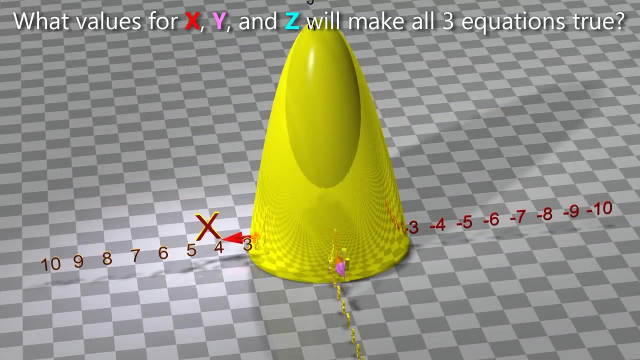 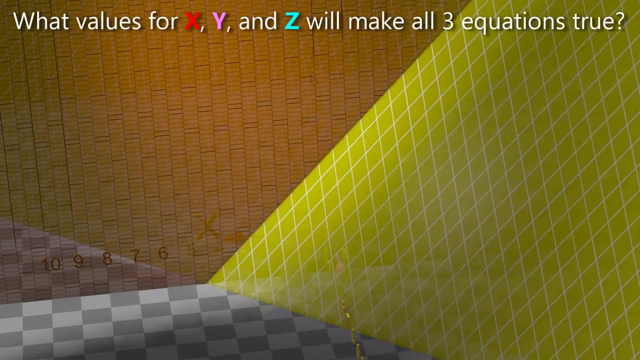 The graph of all the possible solutions looks like this. Now let's look at all three equations at the same time. What values for X, Y and Z will make all three equations true? Points that are solutions to all three equations must be on all three graphs. 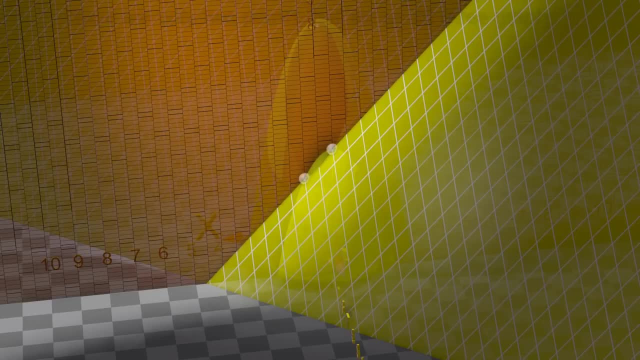 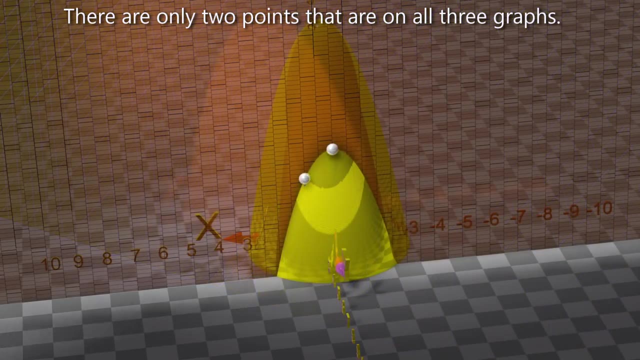 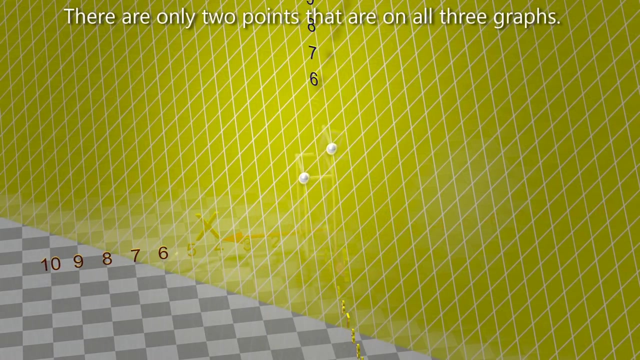 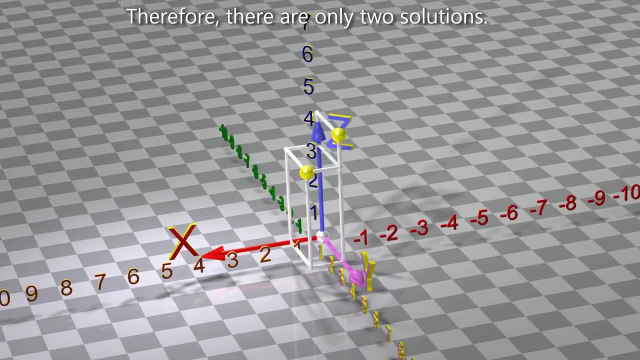 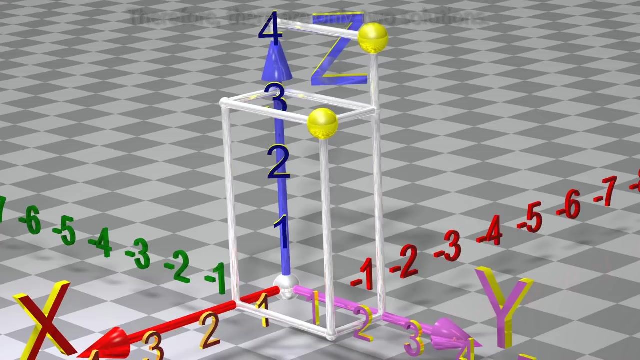 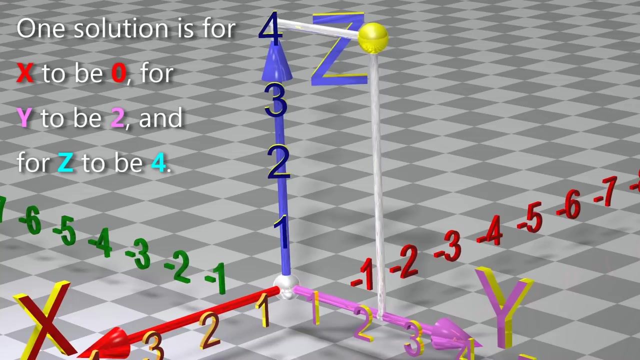 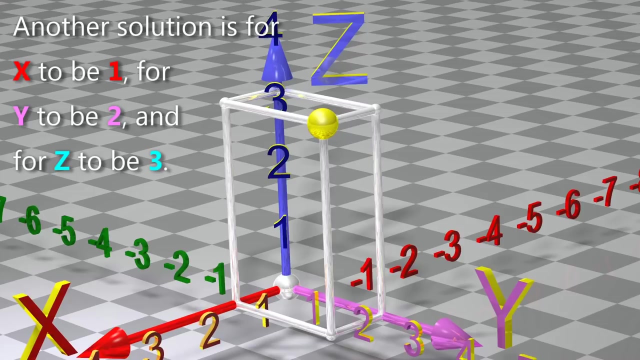 There are only two points that are on all three graphs. Therefore, there are only two solutions. One solution is for X to be 0,, for Y to be 2, and for Z to be 4.. Another solution is for X to be 1,, for Y to be 2, and for Z to be 3.. 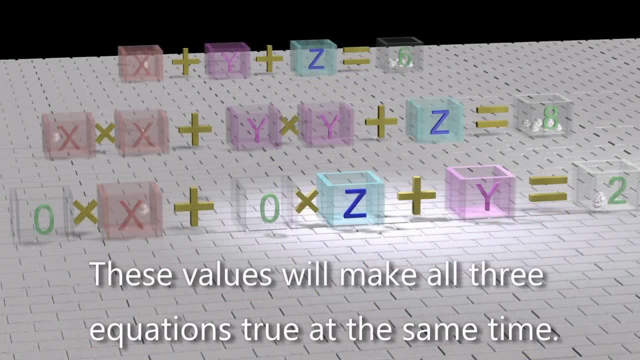 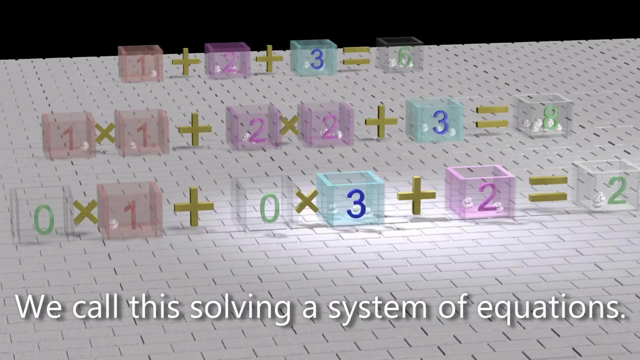 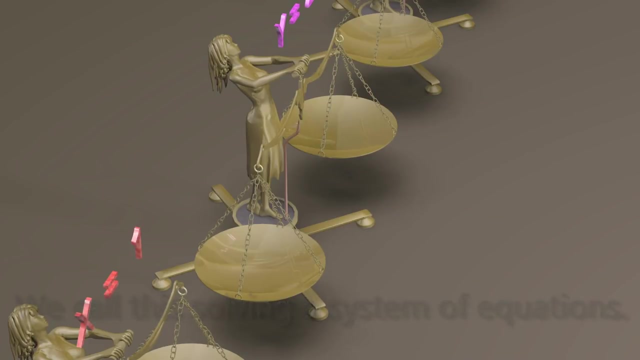 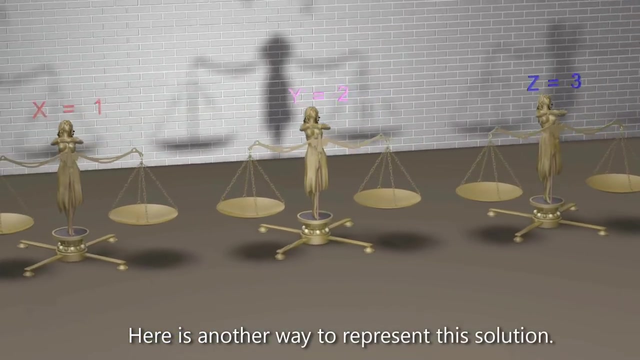 These values will make all three equations true at the same time. We call this solving a system of equations. Did you know that all three equations are real? For example, Z is 0 and Y is 2.. Here is another way to represent this solution. 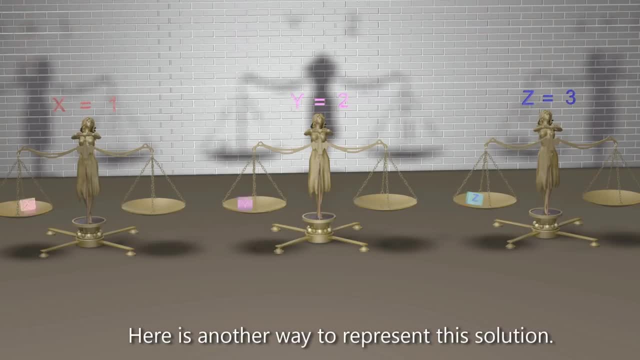 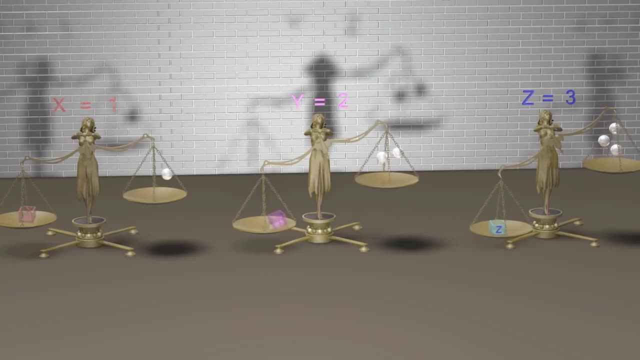 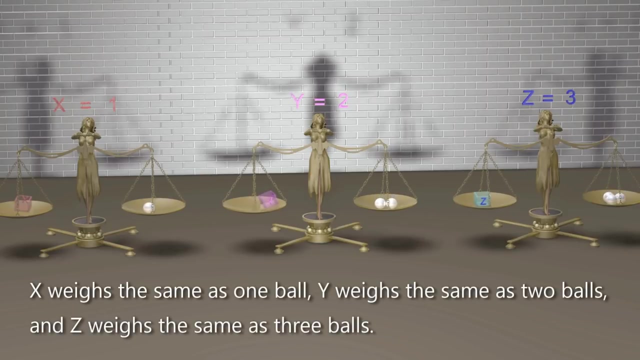 The same is true. with this solution, The value for Y is 1,, for X to be 5, and for Z to be 4.. X weighs the same as one ball, Y weighs the same as two balls and Z weighs the same as. 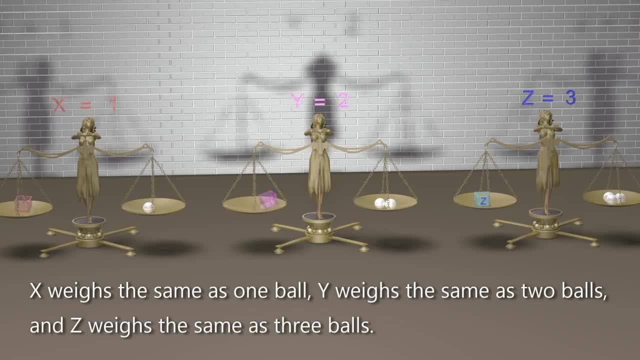 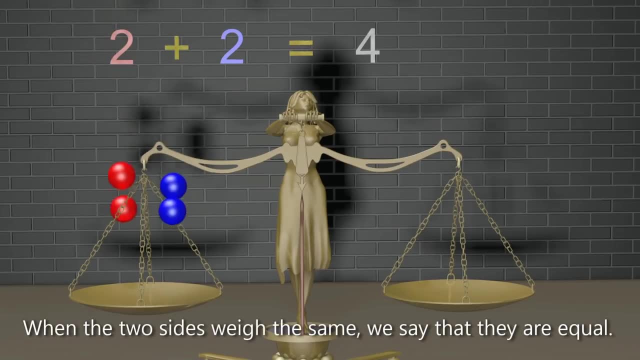 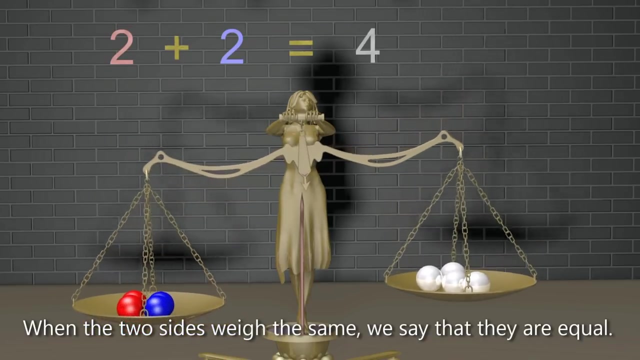 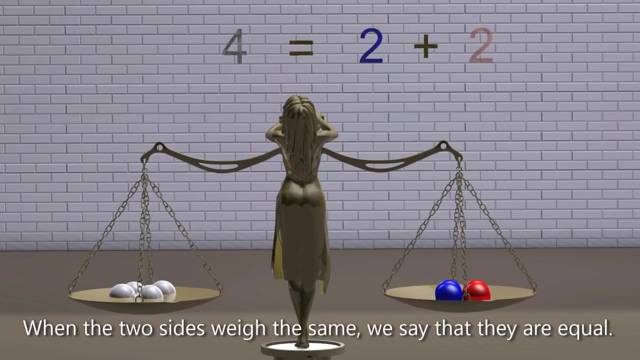 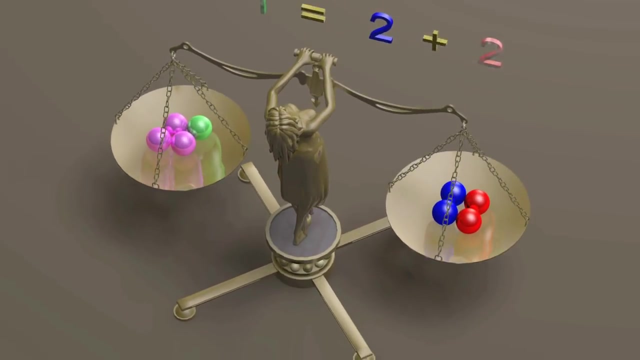 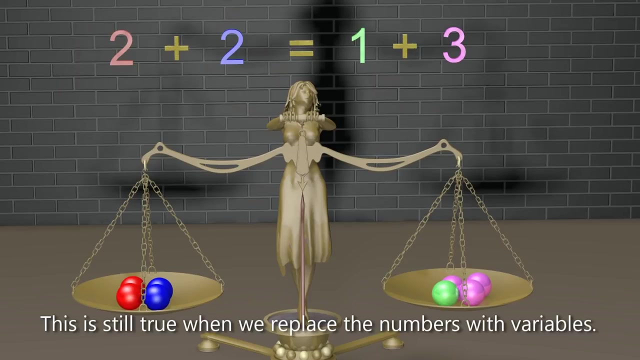 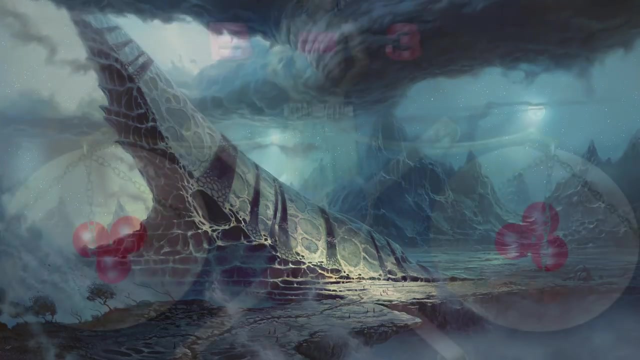 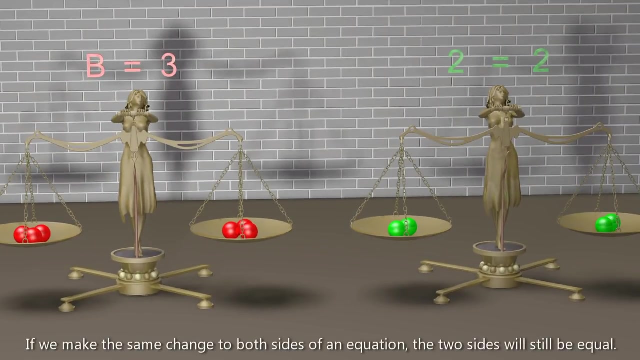 three balls. When the two sides weigh the same, we say that they are equal. This is still true when we replace the numbers with variables. If we make the same change to both sides of an equation, the two sides will still be equal. 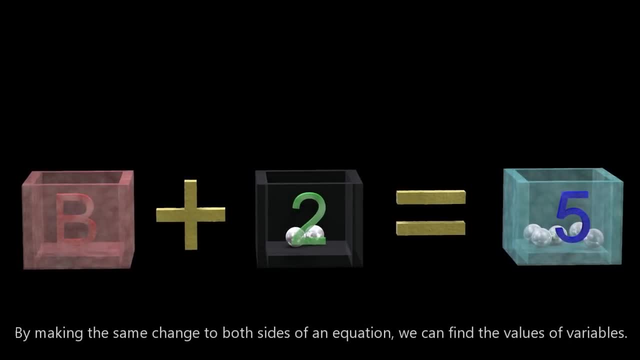 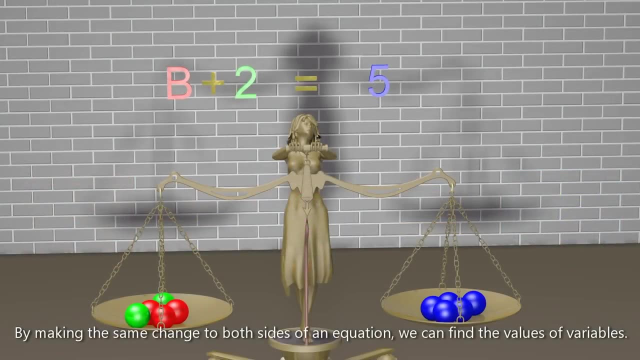 By making the same change to both sides of an equation, we can find the values of variables. If н- the data, d theotes, C the value even, and D- the value for both sides are equal, it well remains und reciprocated. 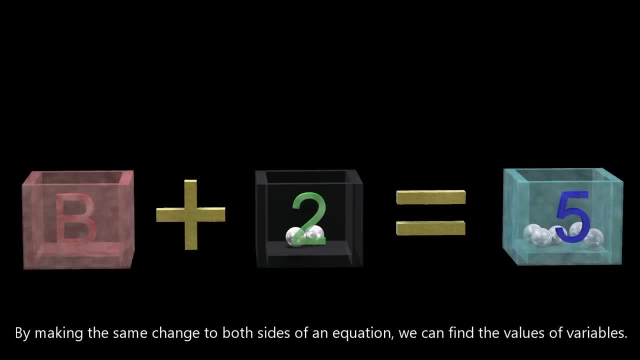 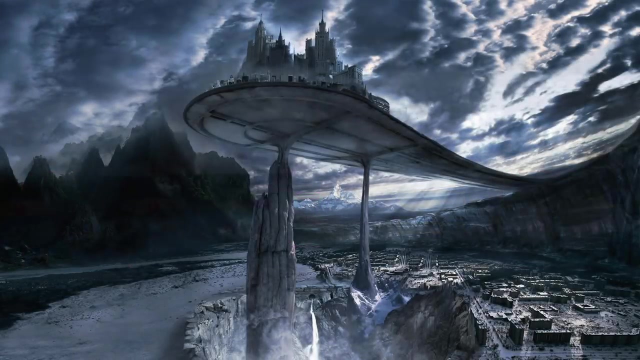 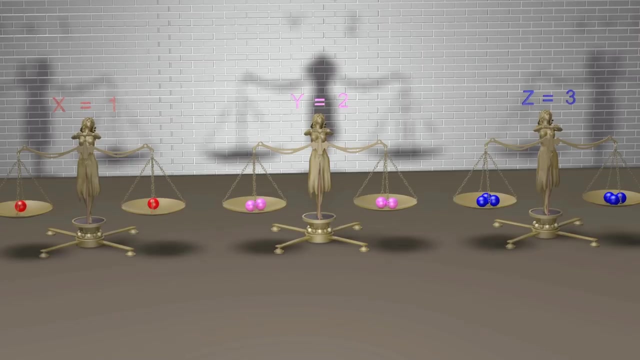 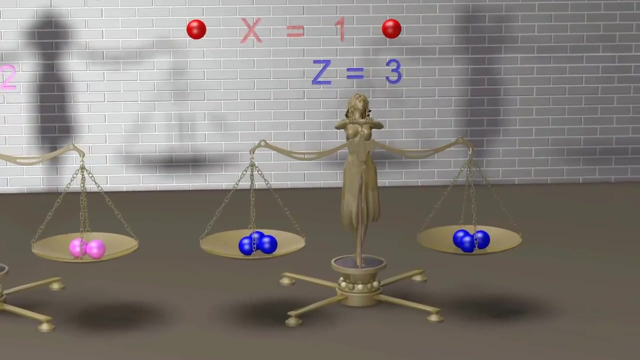 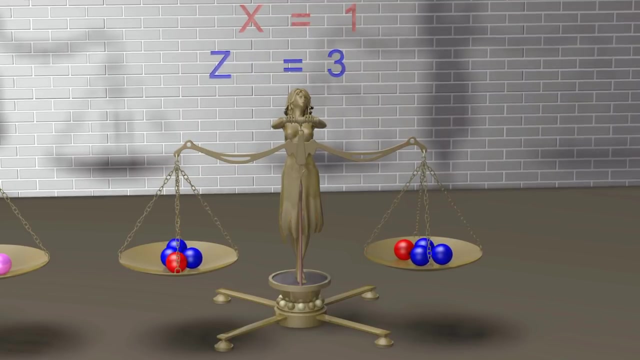 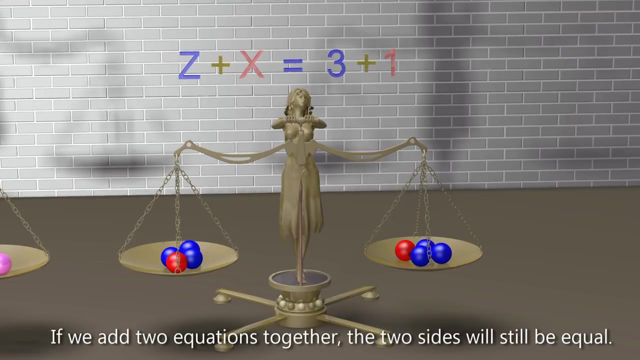 Thus the equation is reversed on the expression that we needed to remove a variance of a matrix. Additionally, when we increase our output on a factor, we have received an angle for each". If we add two equations together, the two sides will still be equal. 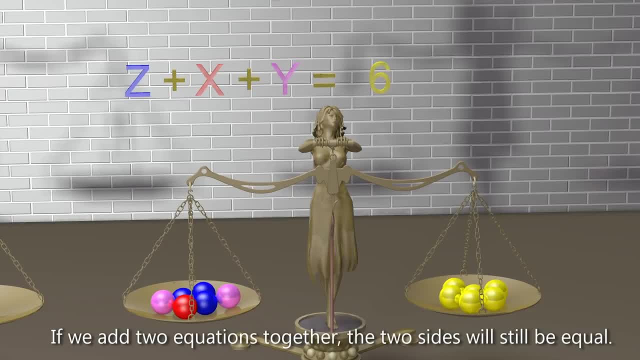 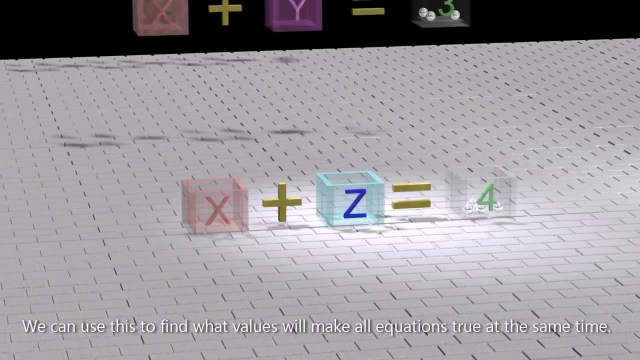 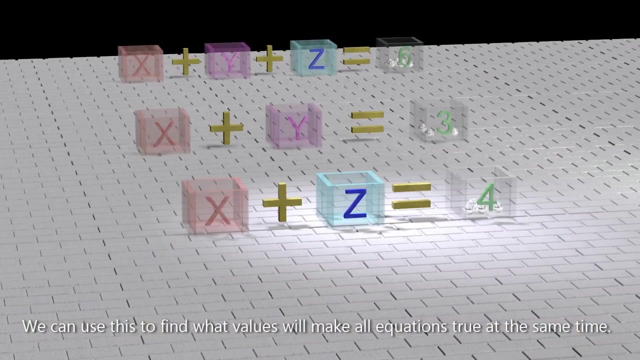 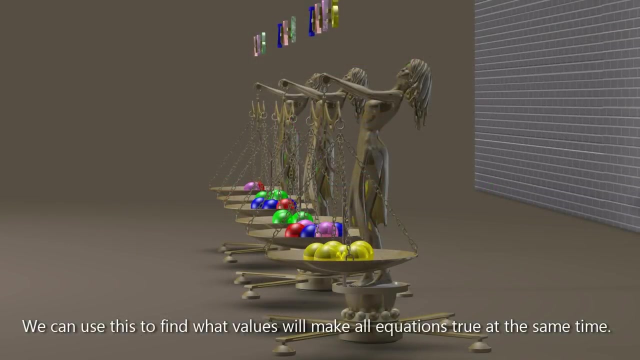 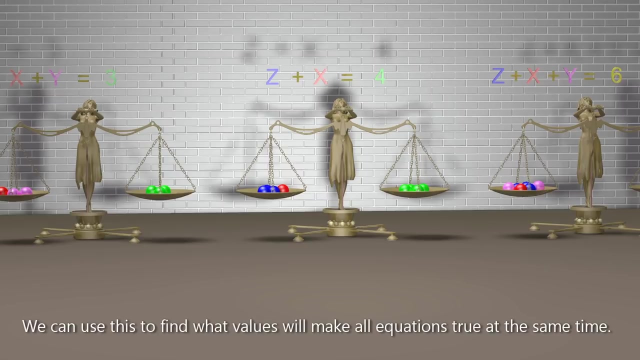 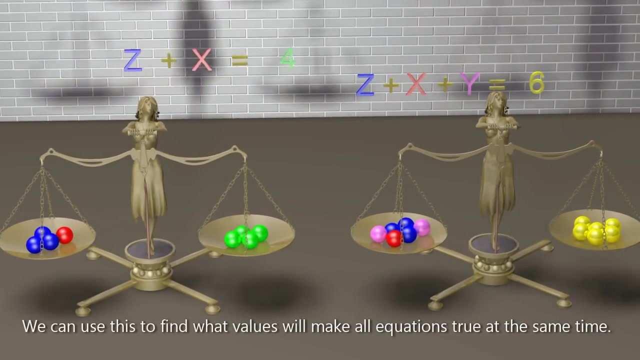 We can use this to find what values will make all the equations true at the same time. We can use this to find what values will make all the equations true at the same time. We can use this to find what values will make all the equations true at the same time. 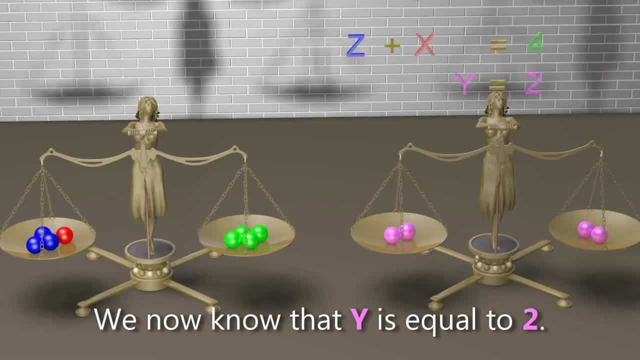 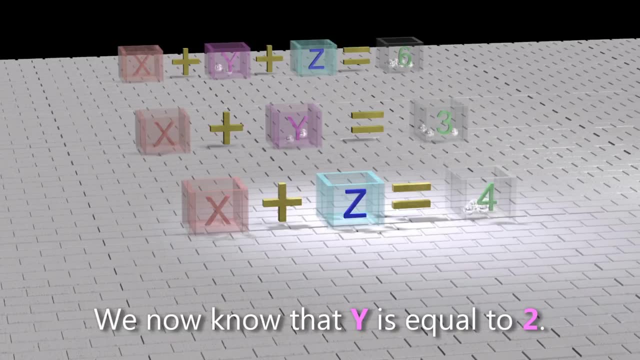 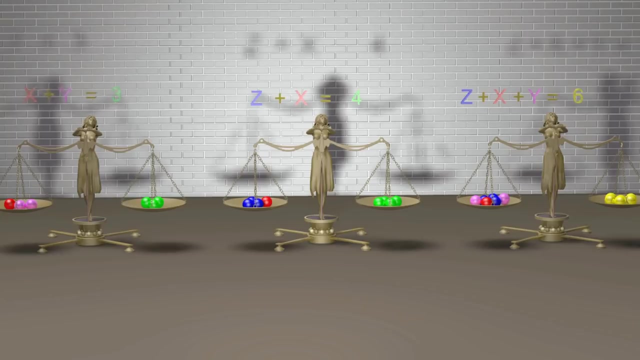 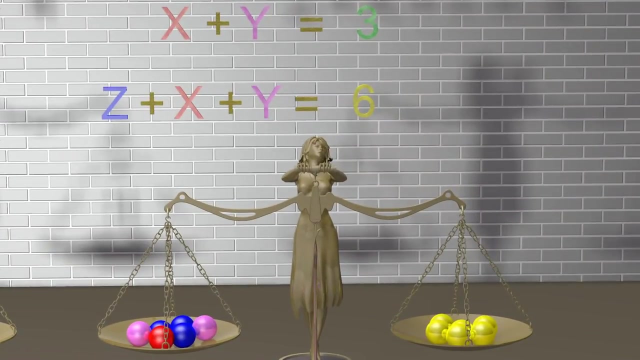 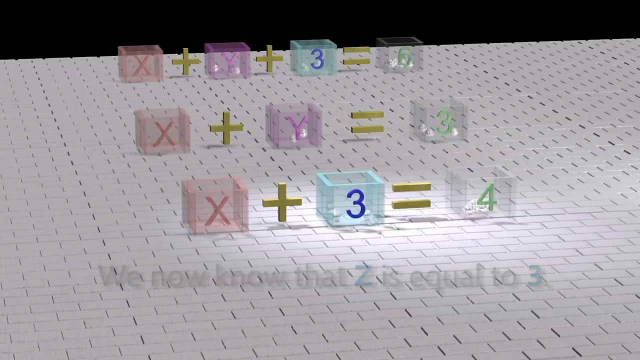 We now know that y is equal to 2.. We now know that y is equal to 2.. We now know that z is equal to 3.. We now know that z is equal to 3.. We previously found that y is equal to 2.. 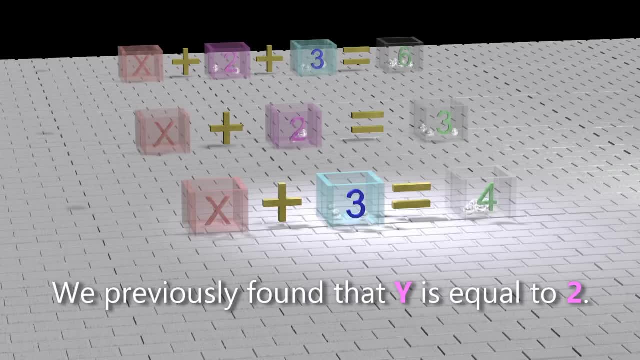 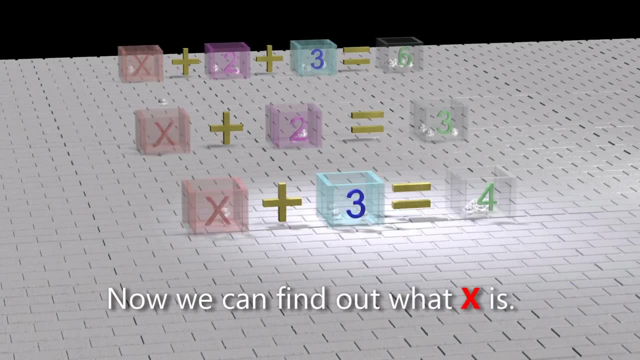 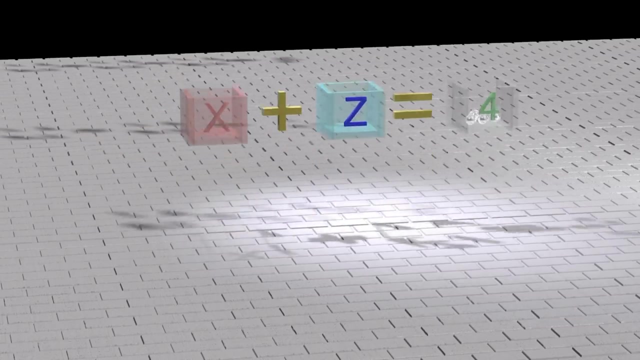 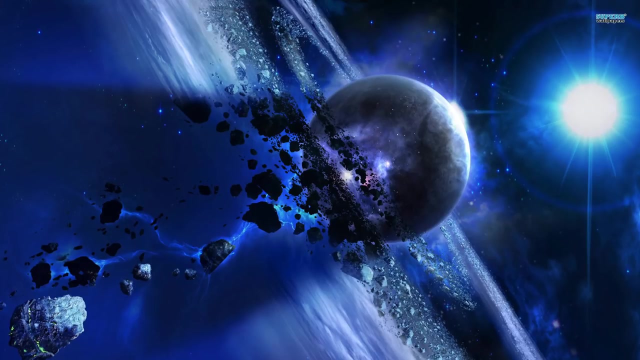 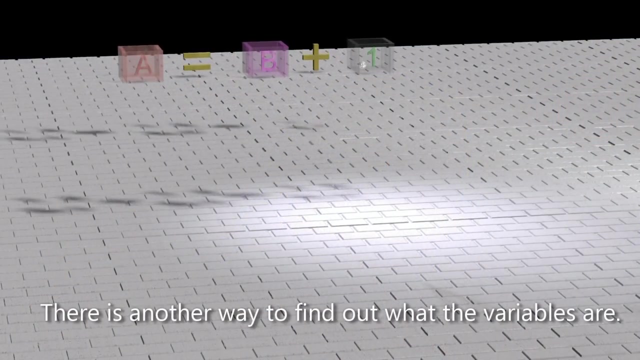 We previously found that y is equal to 2.. Now we can find out what x is equal to 2.. Now we can find out what x is equal to 2.. There's another way to find out what the variables are. There's another way to find out what the variables are. 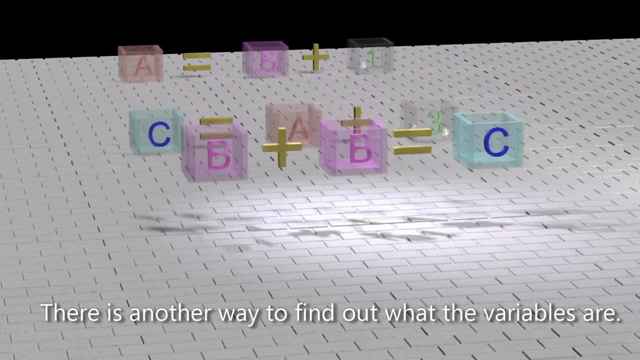 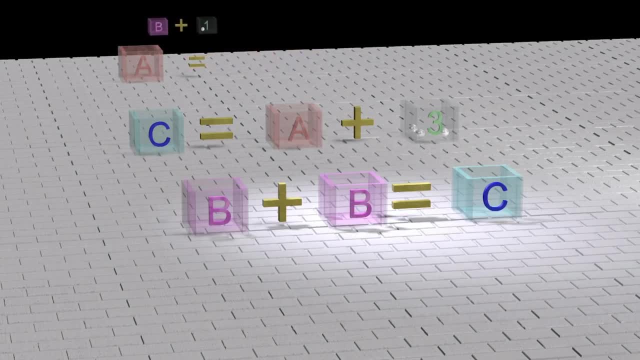 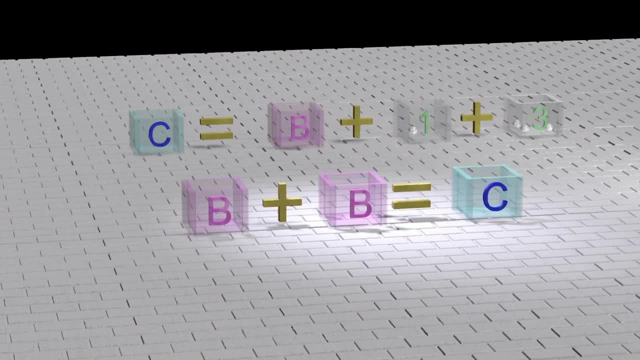 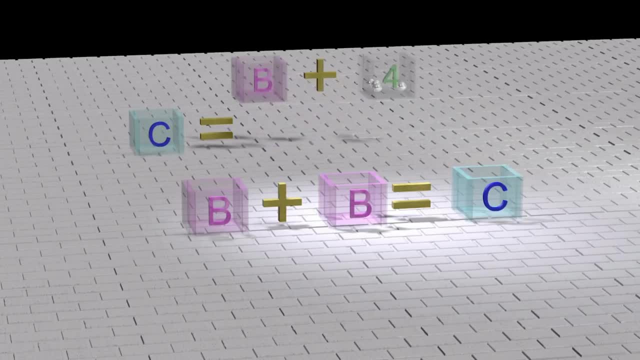 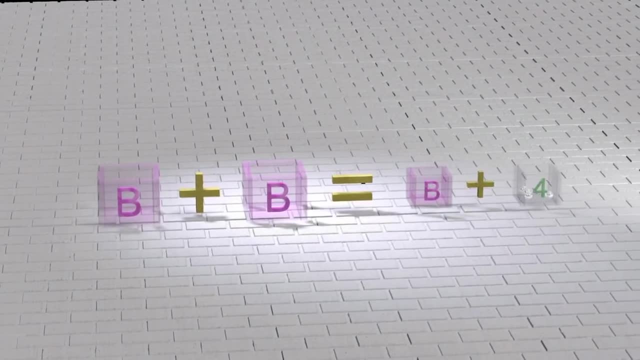 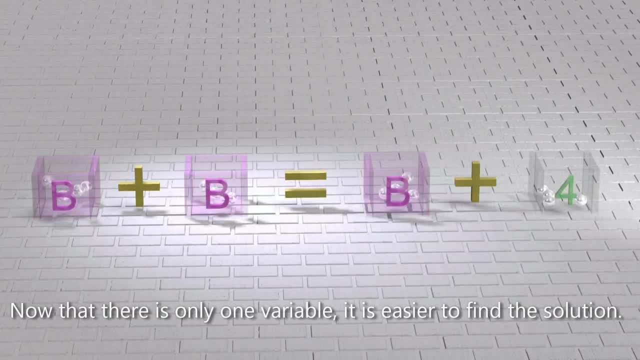 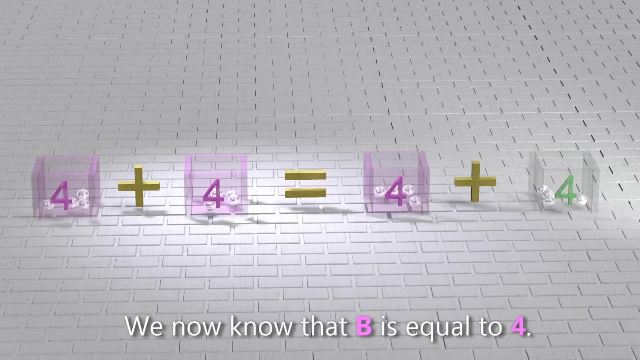 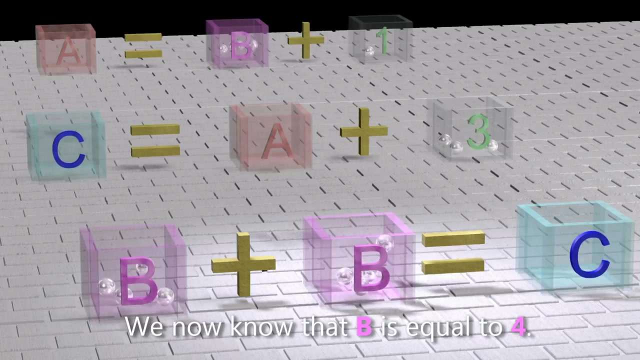 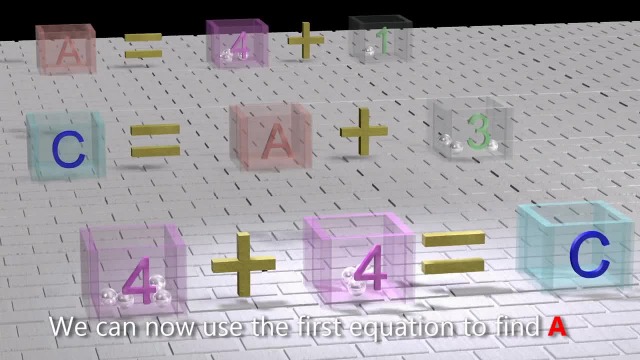 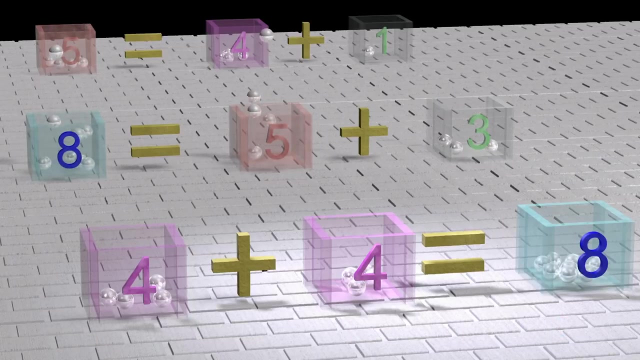 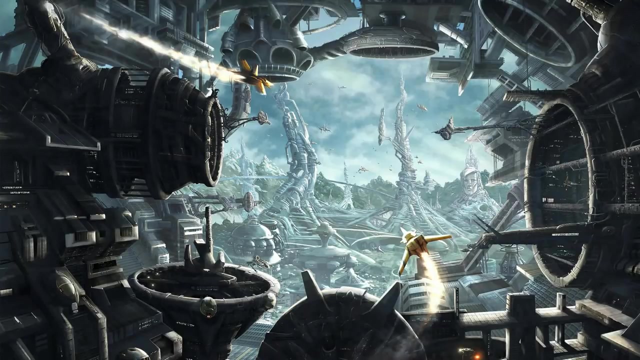 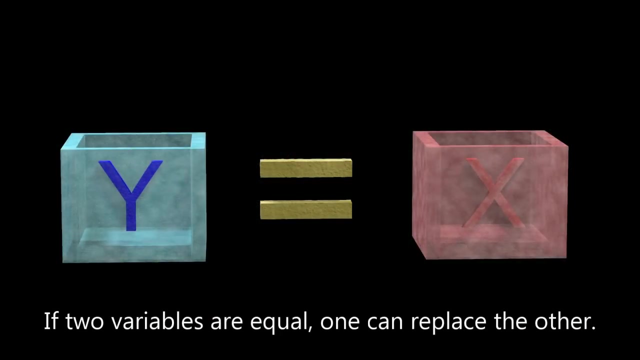 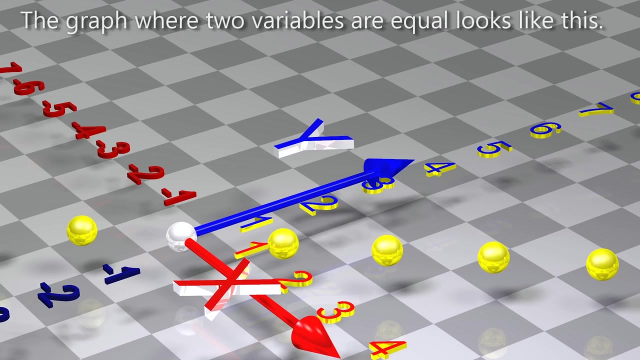 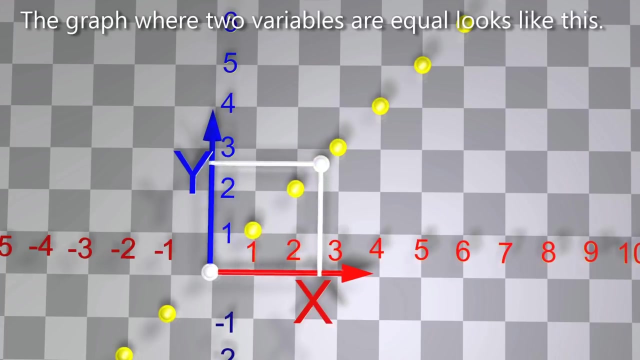 We can now use the first equation to find A And we can use the third equation to find C. If two variables are equal, one can replace the other. The graph where two variables are equal looks like this If the equation is modified: 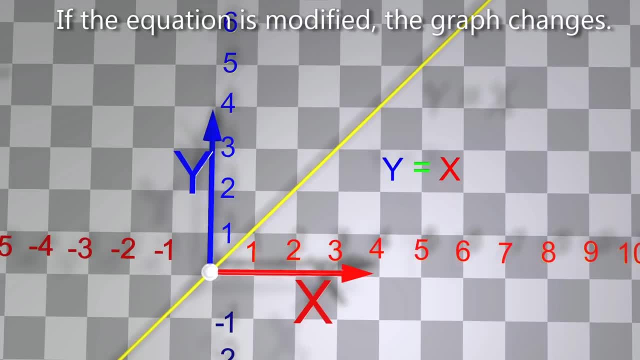 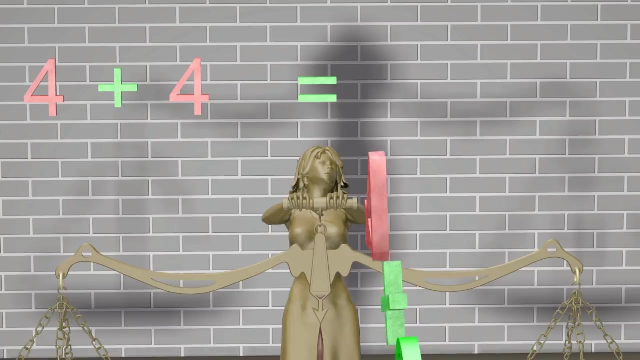 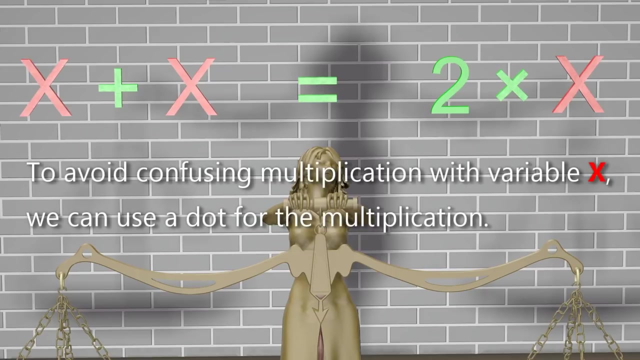 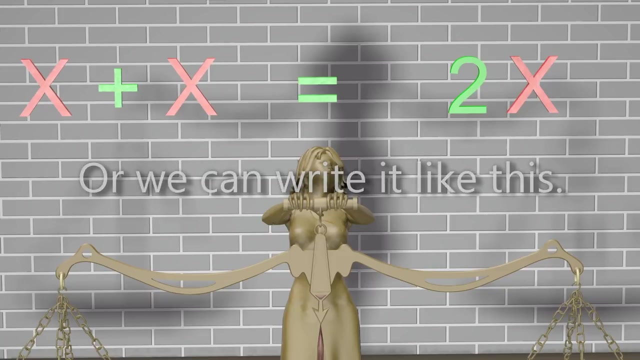 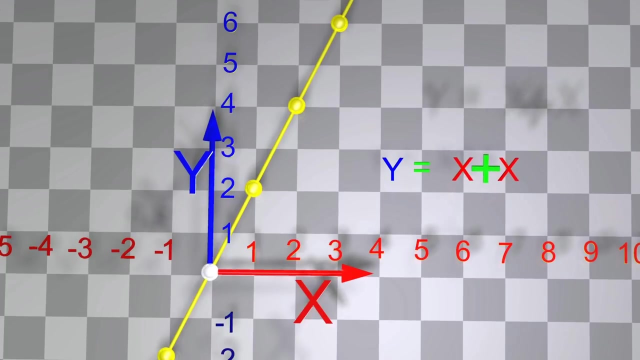 the graph changes. The practicing group can now only find the number of variables. To avoid confusing multiplication with variable X, we can use a dot for the multiplication Or we can write it like this: As the equation is modified, the graph changes. The second green number is where the line intercepts the Y axis. 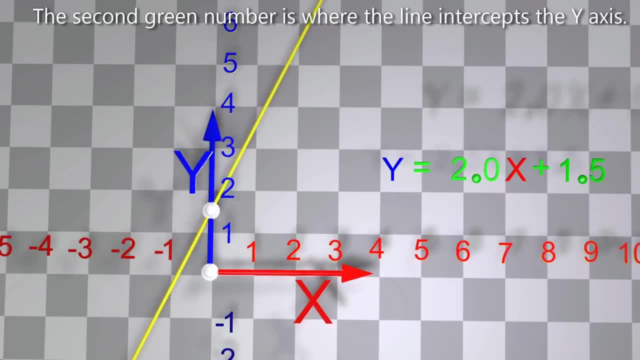 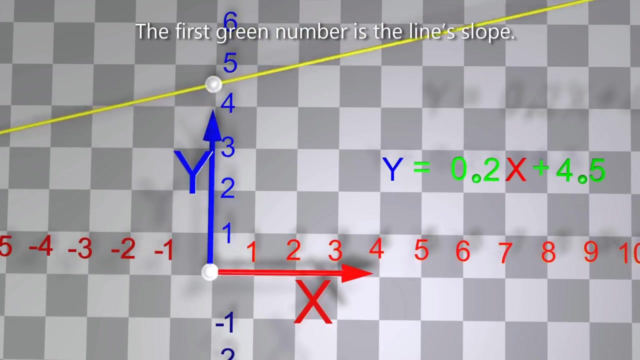 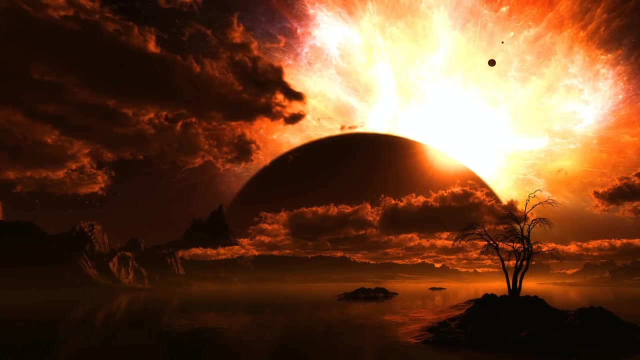 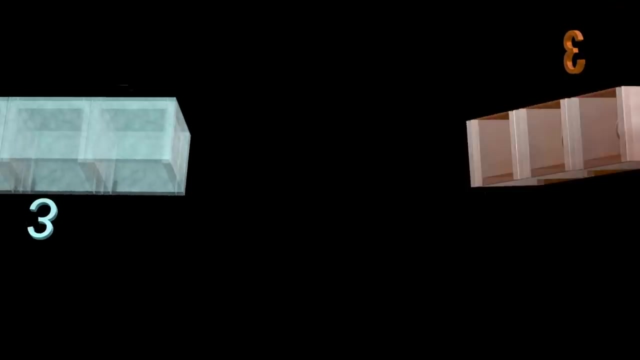 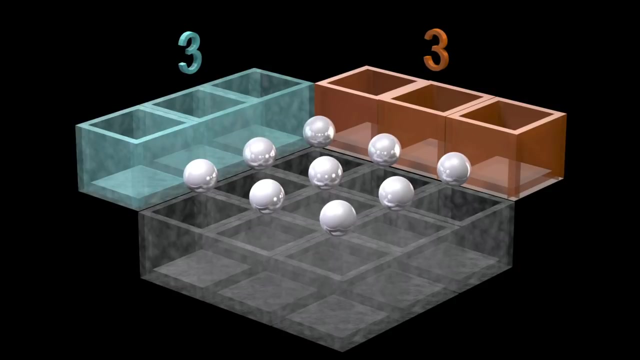 The second green number is where the line intercepts the Y axis. The first green number is where the line intercepts the Y axis. The first green number is the line's slope. The first green number is the line's width. Thank you. 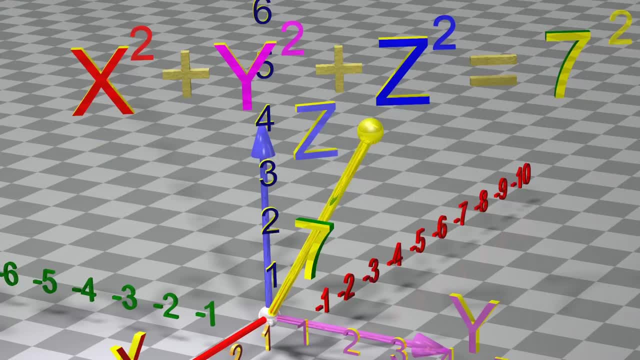 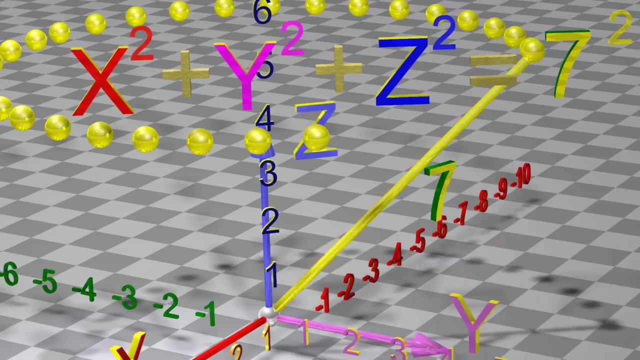 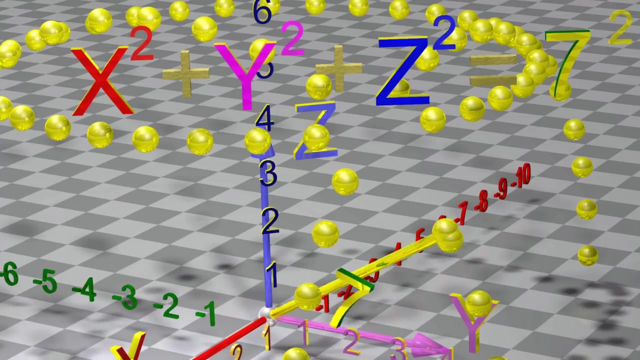 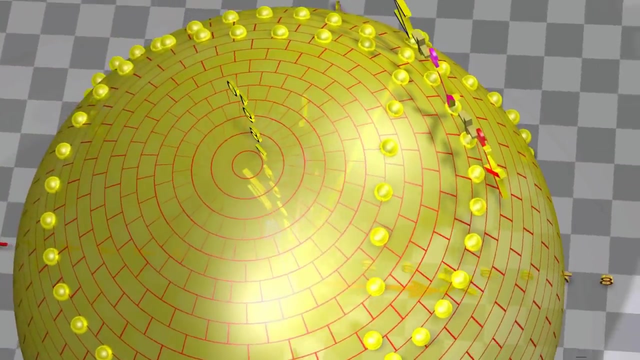 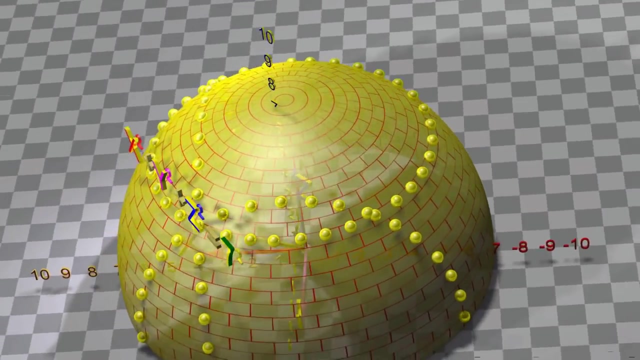 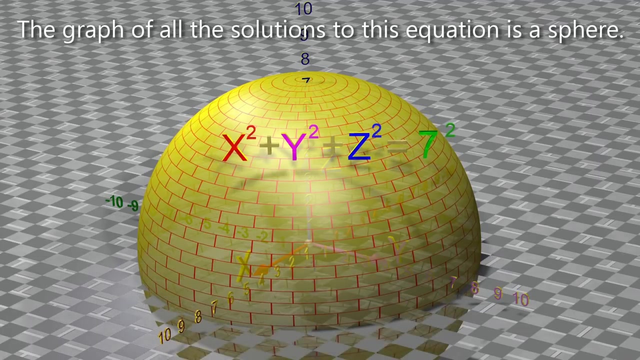 In this case, the distance is 7.. This is the equation for all the points with this distance from the center of the graph. The graph of all the solutions to this equation is a sphere. The graph of all the solutions to this equation is a sphere. 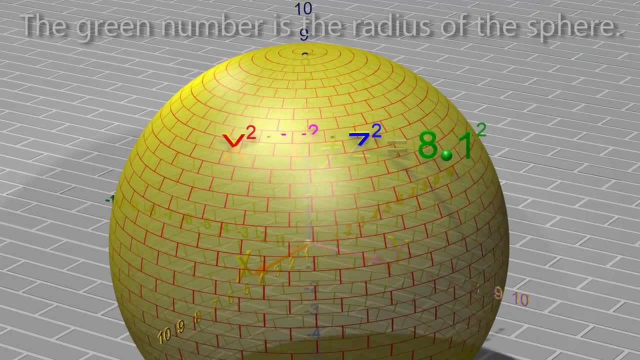 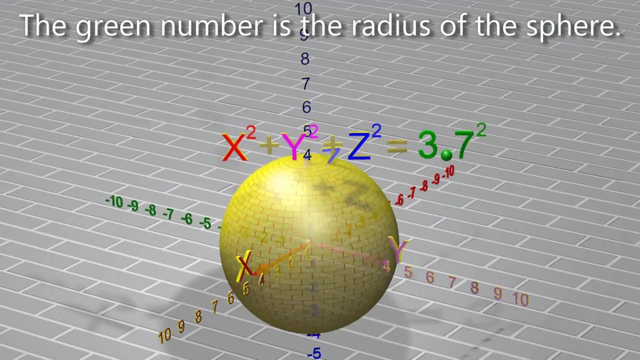 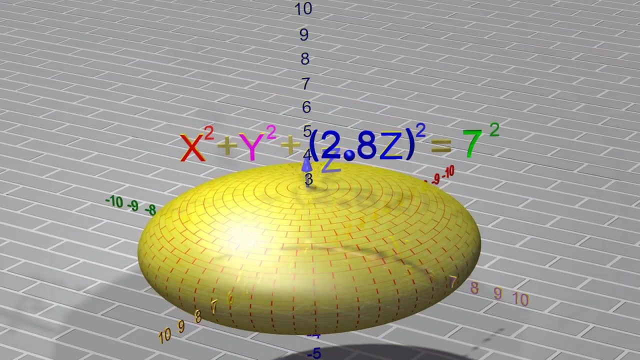 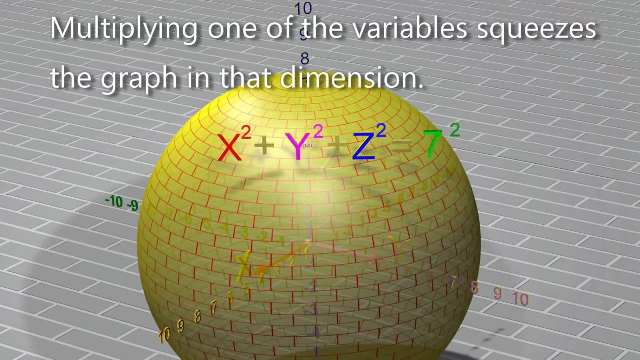 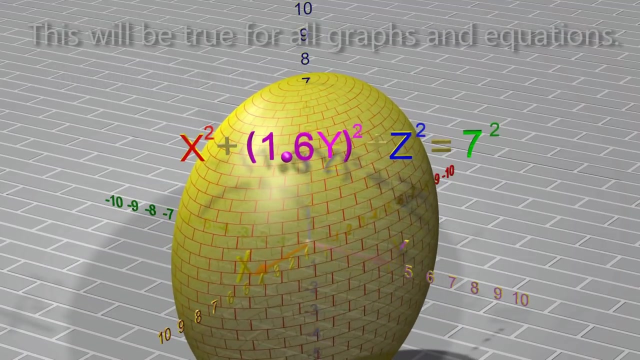 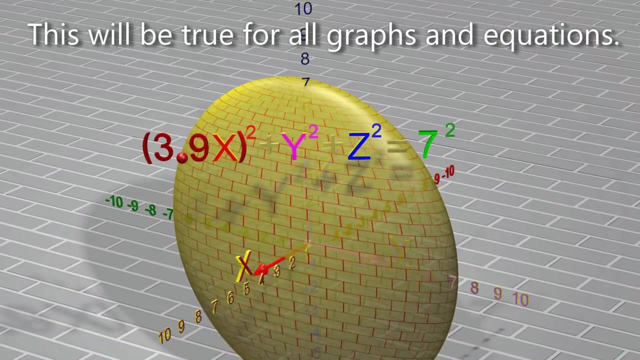 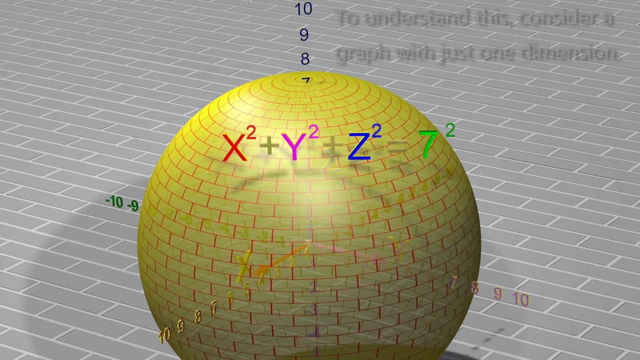 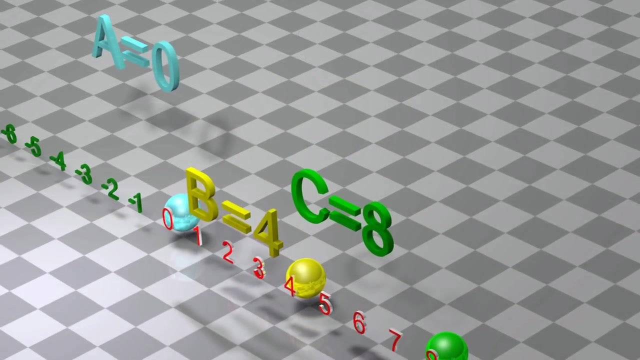 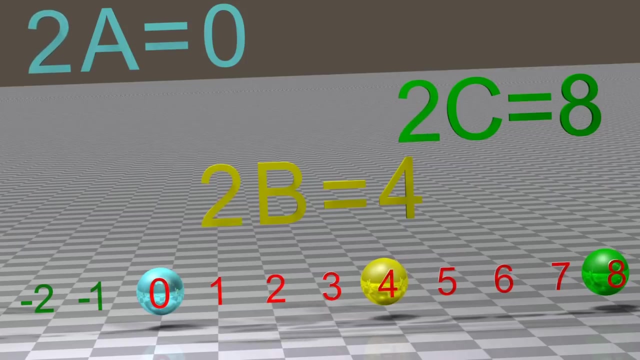 The green number is the radius of the sphere. Multiplying one of the variables squeezes the graph in that dimension. This will be true for all graphs and equations. To understand why this happens, consider a graph with just one dimension To understand why this happens. 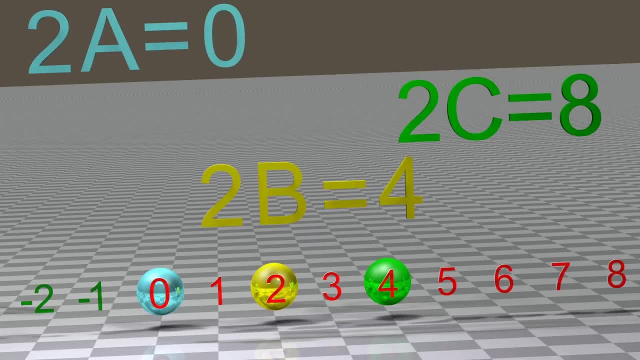 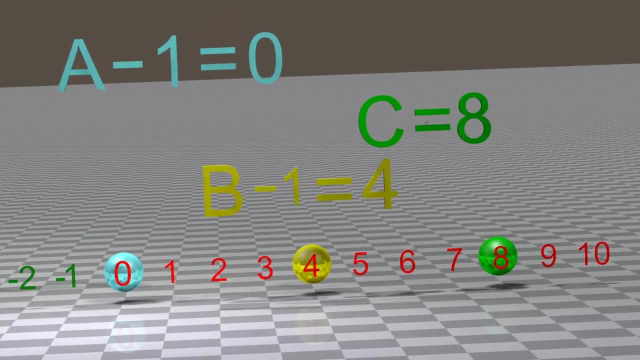 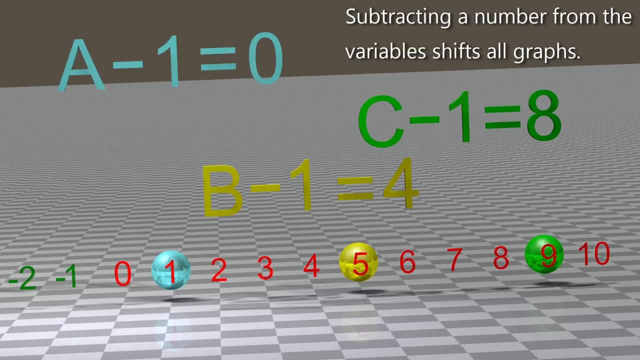 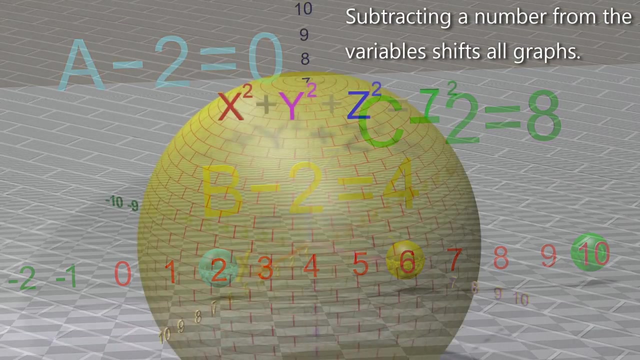 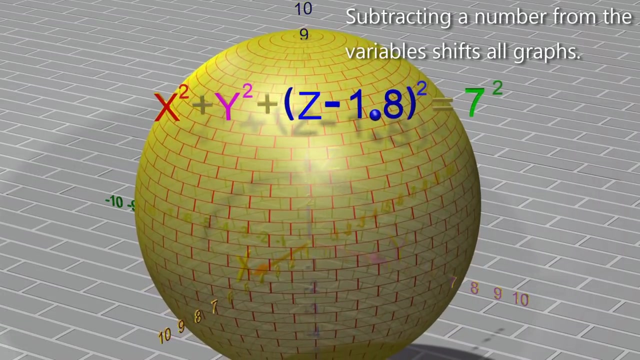 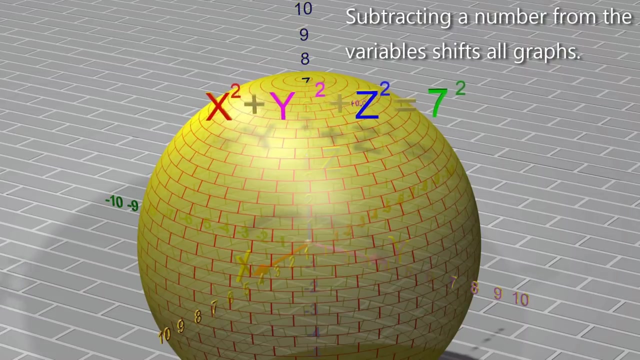 consider a graph with just one dimension To understand why this happens. consider a graph with just one dimension. The solutions to the equations are now squished together. Subtracting a number from the variables shifts all graphs: Ft, Ft, ff², ff². 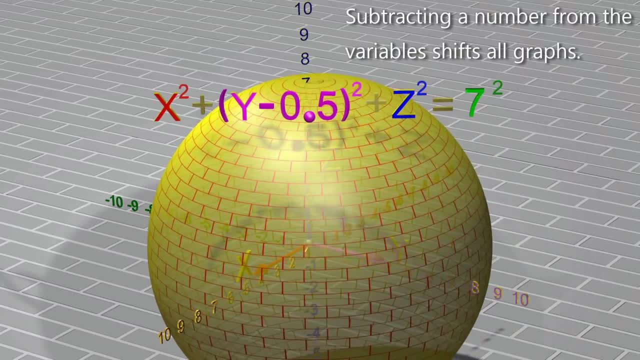 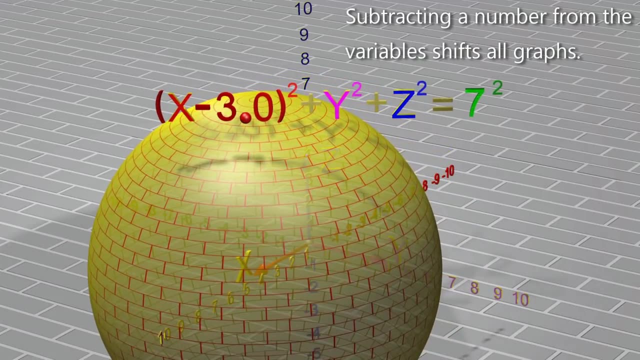 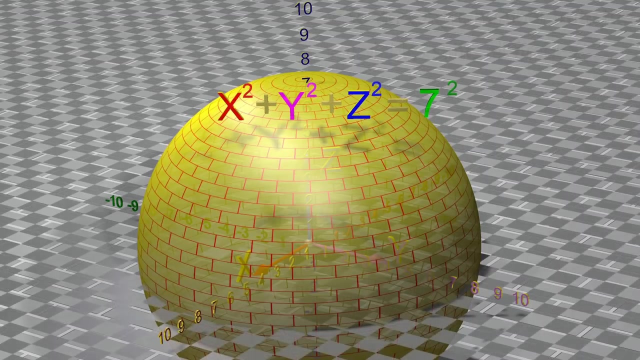 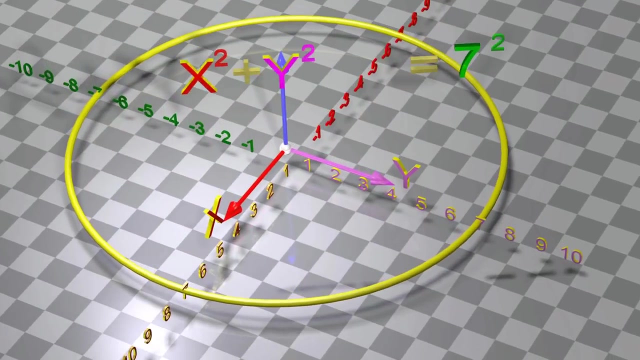 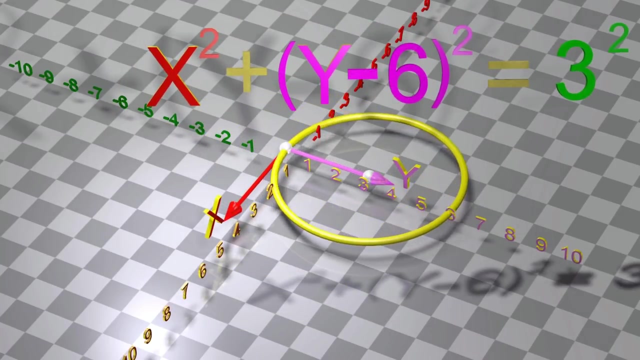 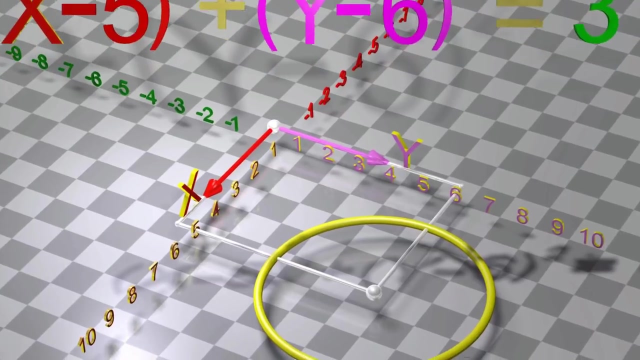 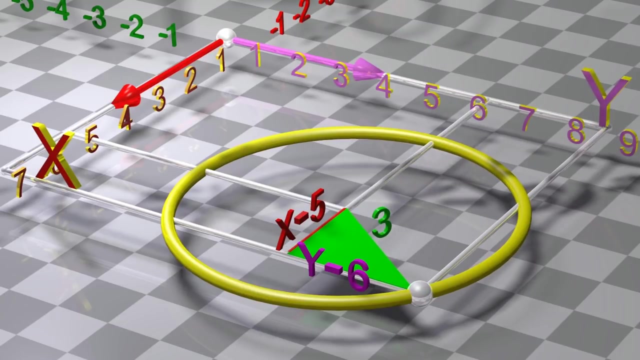 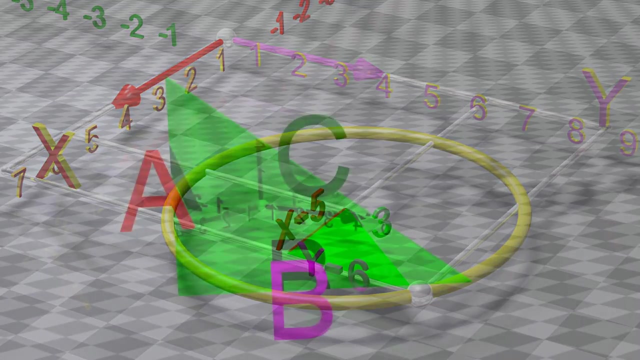 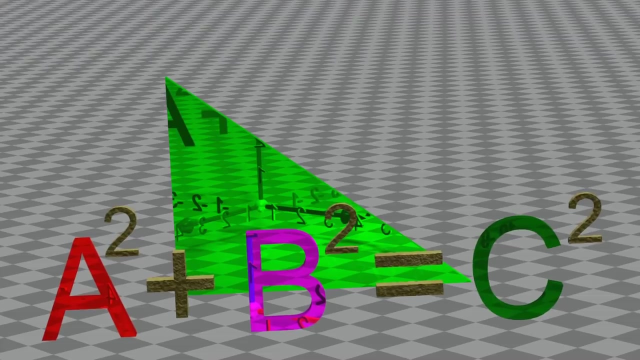 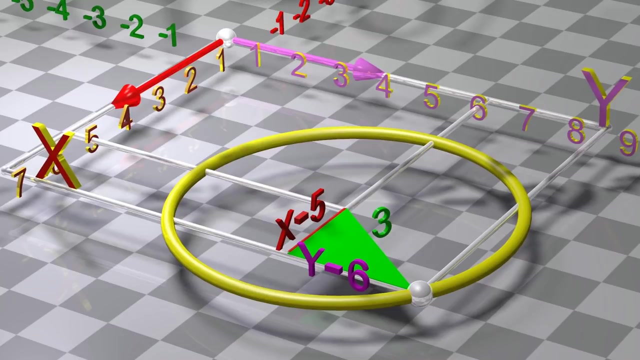 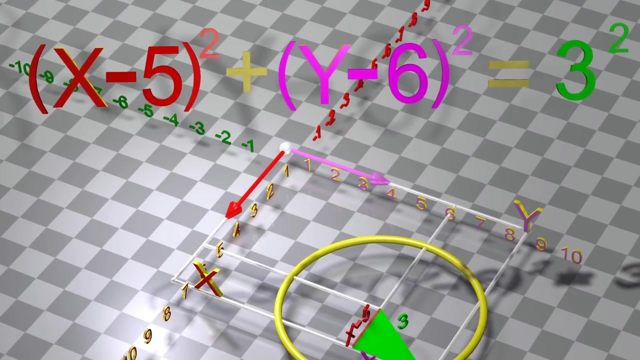 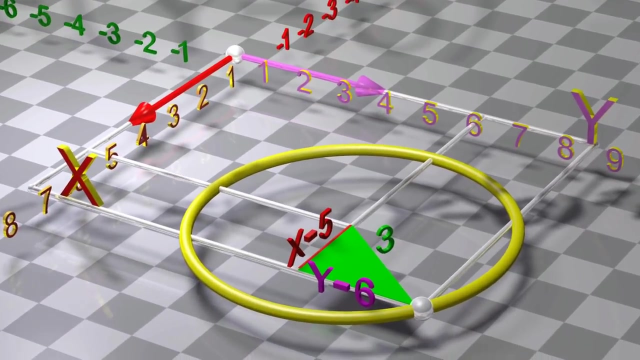 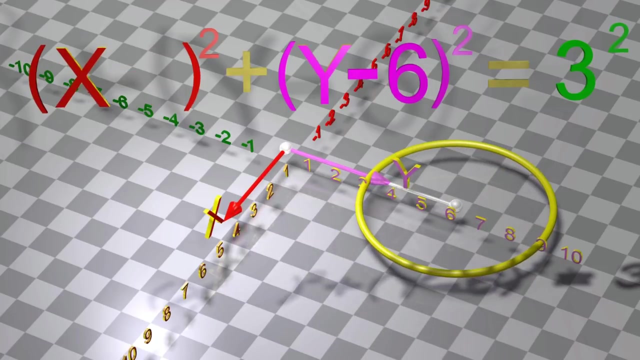 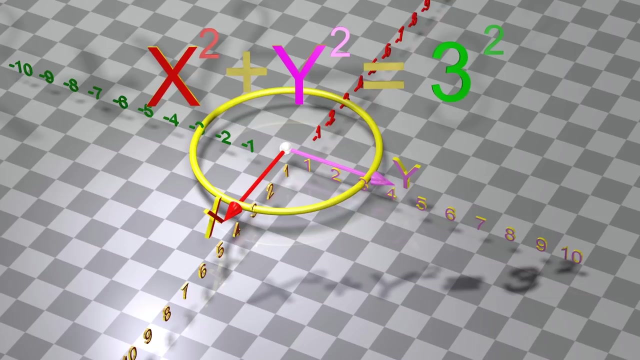 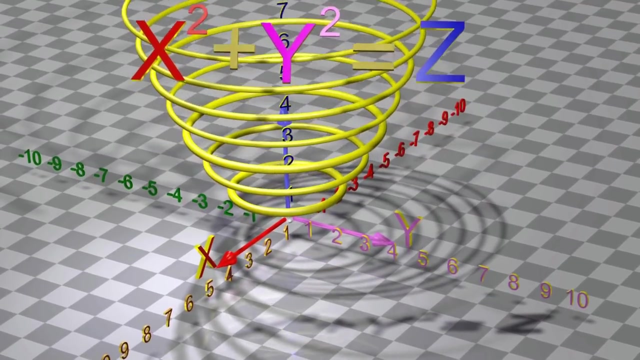 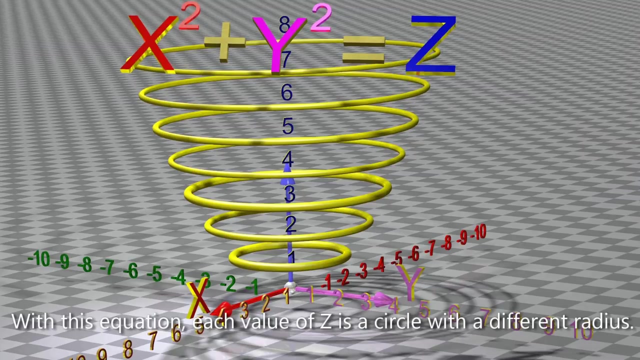 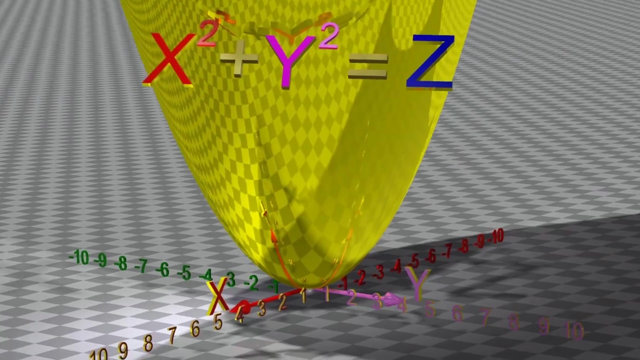 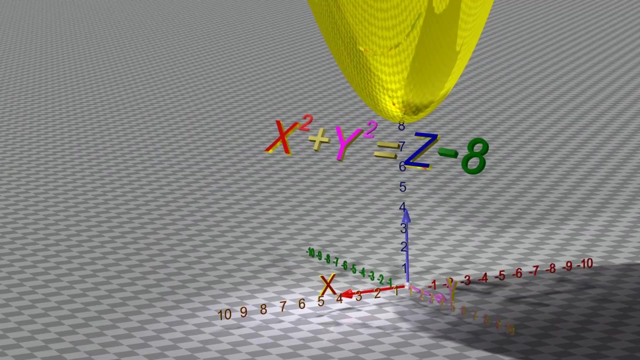 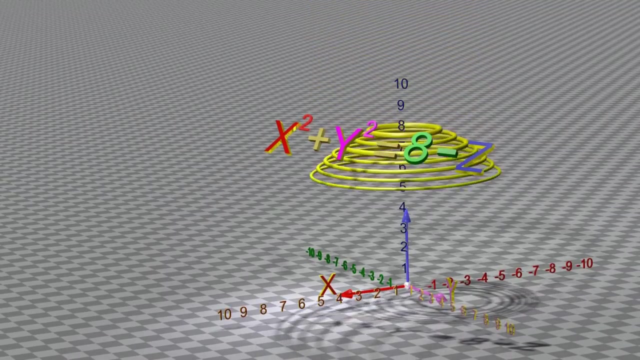 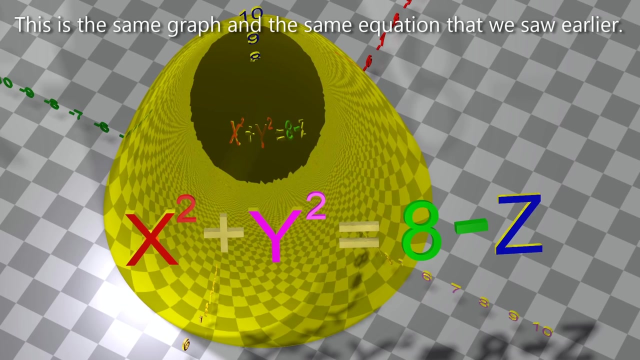 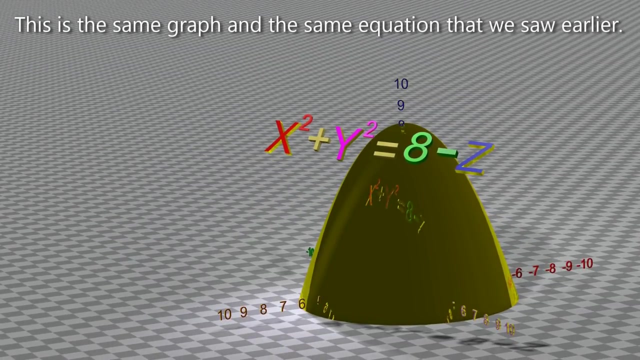 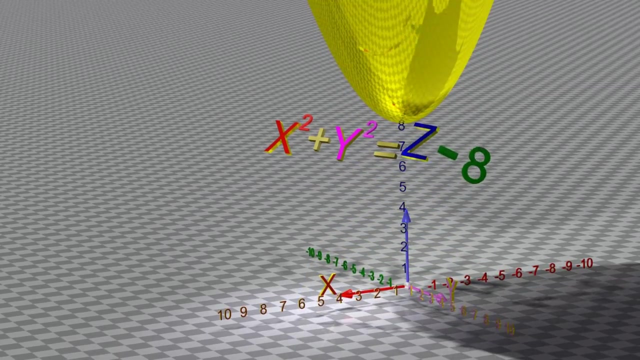 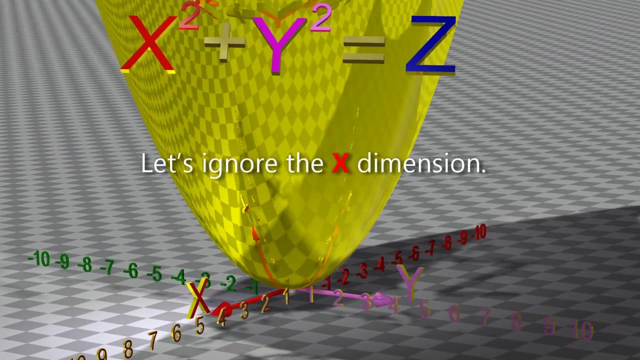 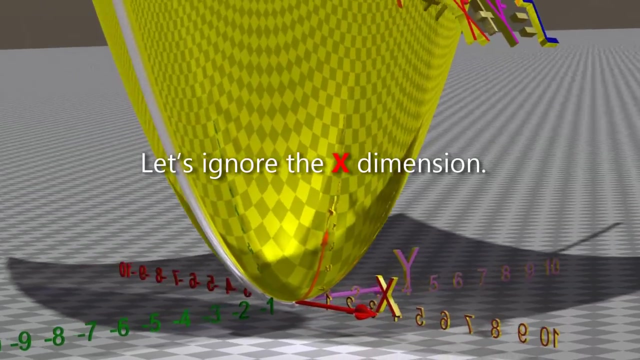 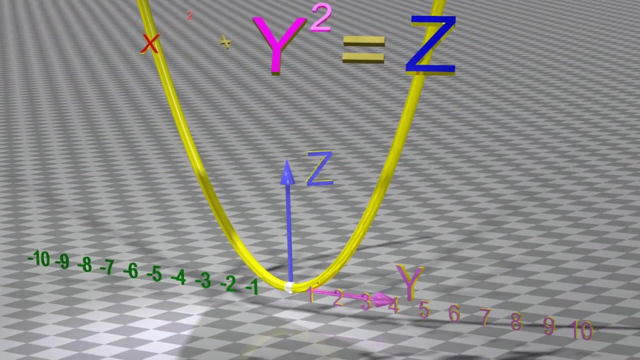 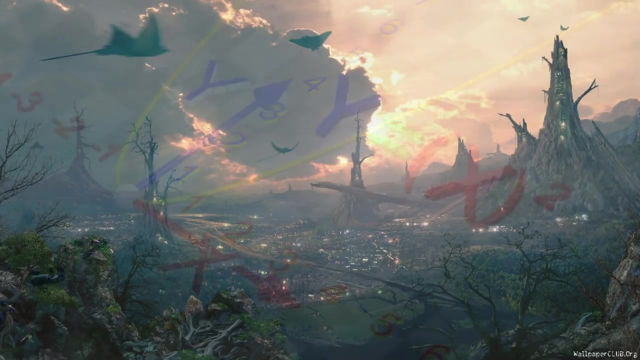 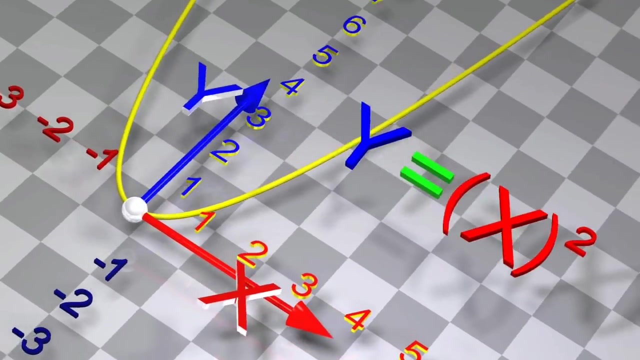 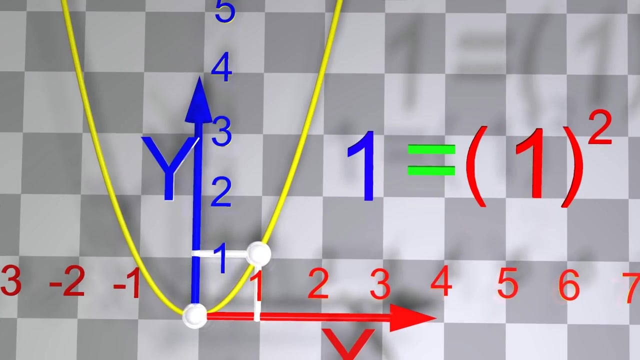